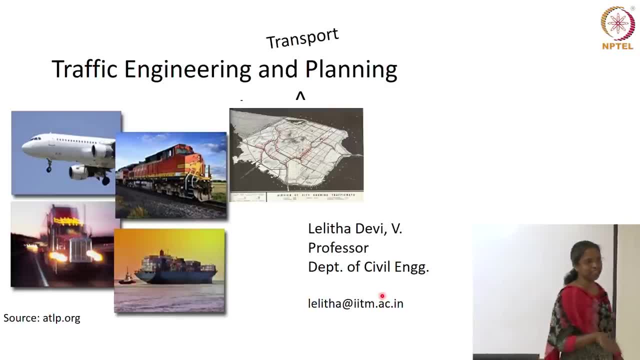 So let us, let us move on. So what is traffic engineering? is they will edit whatever they do not want from here? So what is traffic engineering, as per your understanding? I need answers, there is no way, otherwise I cannot read Traffic engineers. Ok, but that what? 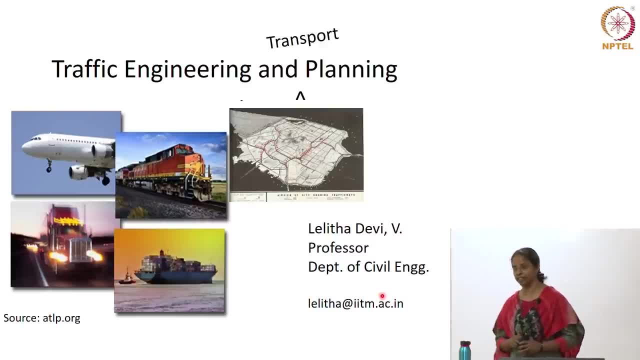 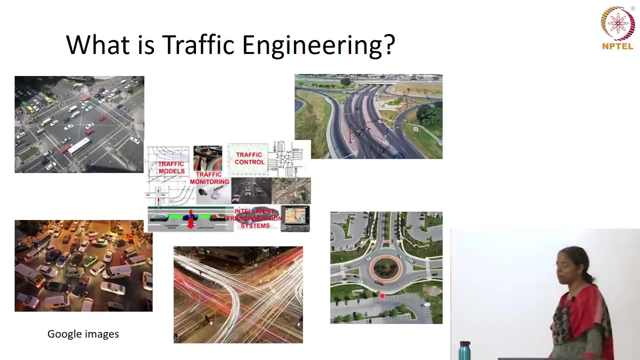 is that life cycle includes different traffic engineering. So traffic engineers, they have different tasks. Before construction, there is one more thing: yes, planning, then construction. Ok, good, you looked at the slides, I guess: Ok, ok, let us come back, come back. So stop, stop, stop. So this is what I got when I 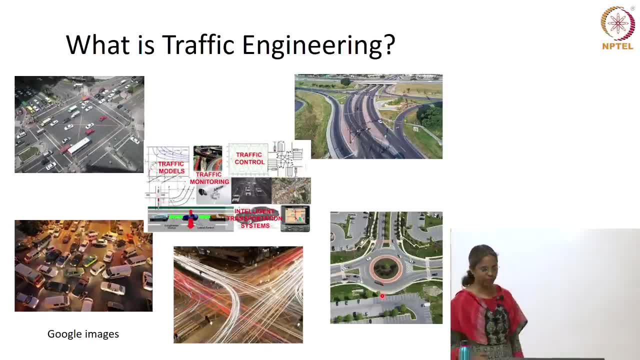 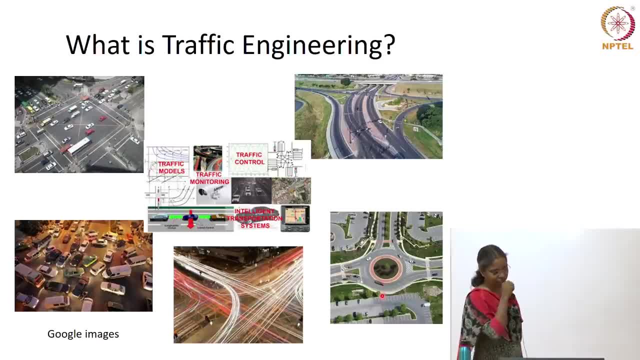 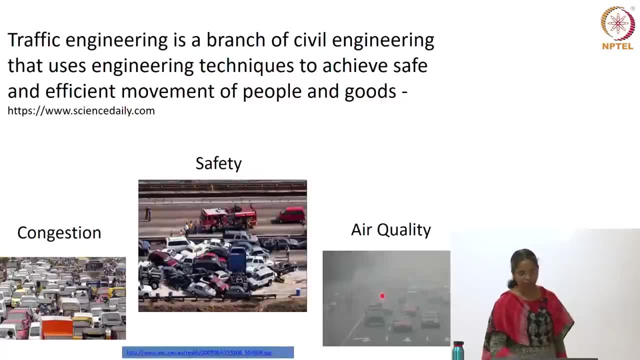 models, traffic control, traffic monitoring, intelligent transportation systems. So all these are covered by what he said is what I believe. So let me look at, show you the simplest definition I saw in a website, which is a very simple website. It says: traffic engineering is a branch of civil engineering that uses engineering. 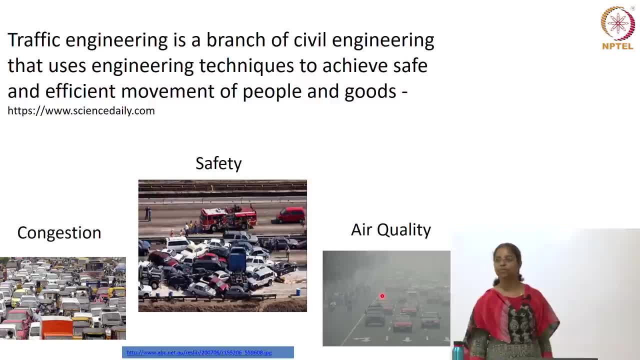 techniques to achieve safe and efficient movement of people and goods. Very simple, right, And it conveys what traffic engineering is all about. It is all about moving people and goods from one place to another. The major conditions that you add is safe, efficient. 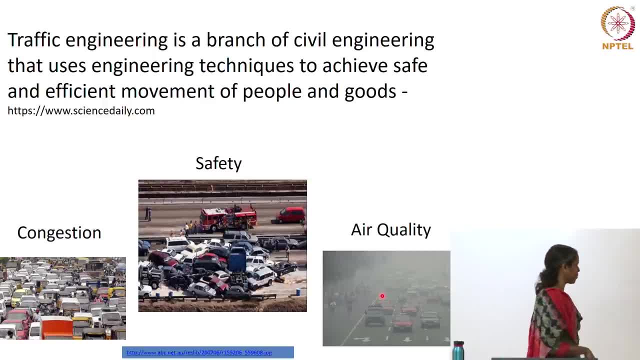 and economic movement. So this is what the traffic engineering is, And why do we do this? There are mainly three problems which we talk about. One is congestion, the other is safety, the third is pollution or, you know, emission. So when you say we 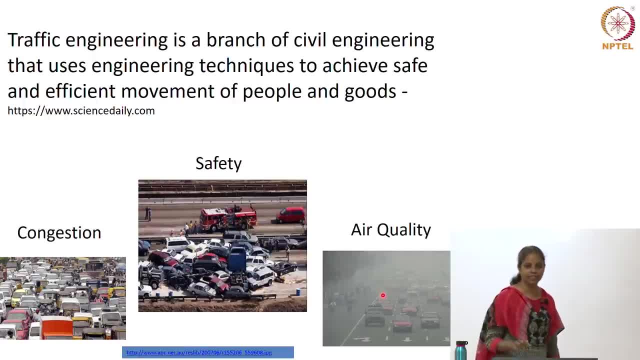 have to design this system we are talking about. how do we address these problems or design the thing such that these problems are minimized? And what is the problem here? when you are trying to minimize some of these, or when you look at these objectives, you 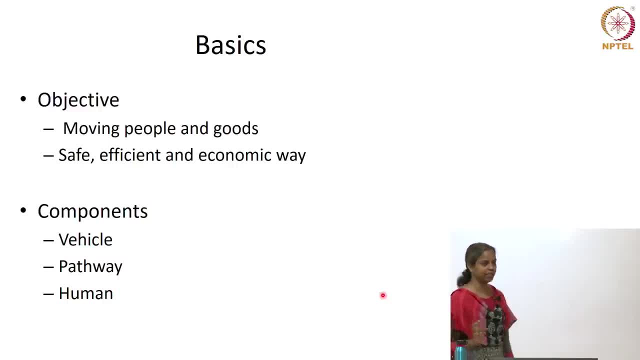 will see the basic objectives. Let me go to the next slide. So the basic objectives you will see in any. anywhere you read is the like: safe, efficient and economic movement of people and goods. So what is the problem here? I have a problem in these three objectives. 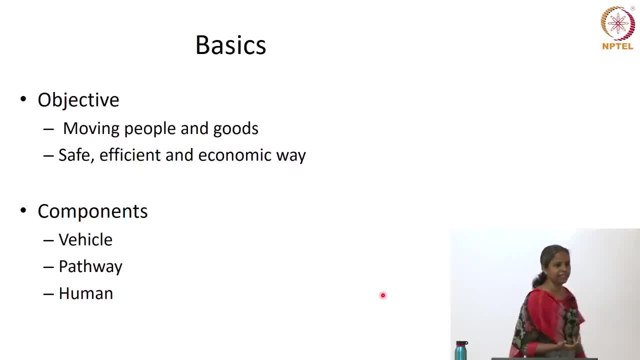 that we are talking about. ok, When you talk about safe, how do we make a traffic system safe? So usually you talk about reducing speed. right, That is how you talk: make it more safe. But then if you want to make it more efficient, what should you do? You have to make the move. 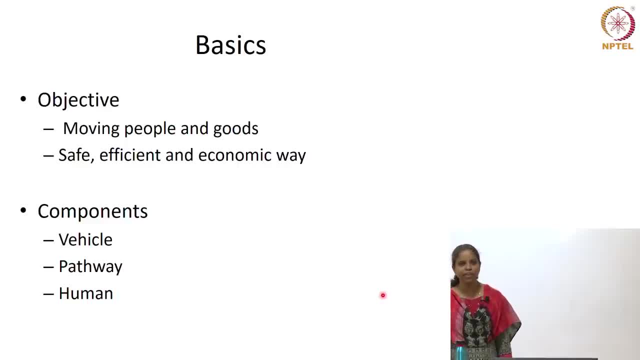 as fast as possible, right, So we are seeing some conflicting objectives in the whole process. That is the difficulty. So we always look for the optimum way of handling these problems. How do we make them move fast enough and safe enough? But it is again. you cannot say that. 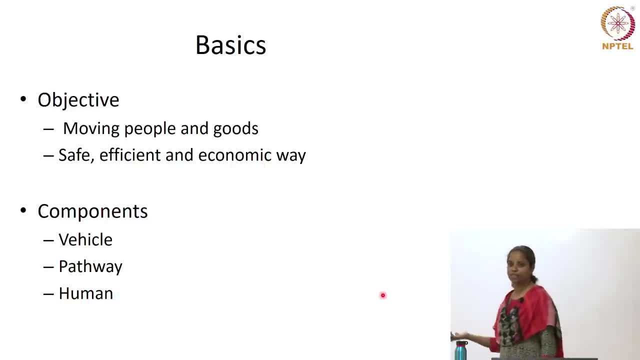 average is good enough. We want the minimum excellence. So we cannot say 50 percent of the traffic is safe, So we have to make the traffic as fast as possible. So we have to make the traffic as fast as possible. We have to make the traffic as good as possible. But 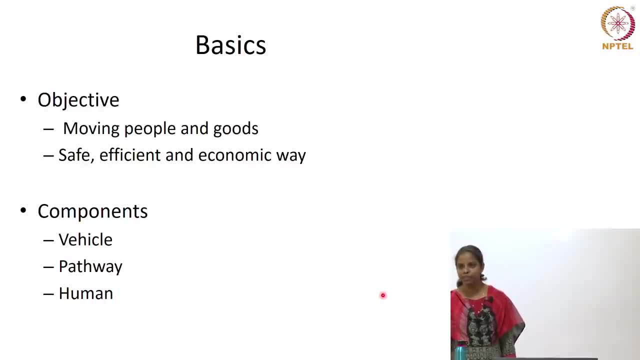 we cannot say that this is good enough for you. So that is one of the major challenges you will face when you are trying to do this. And what are all the components that we are talking about? There are mainly three components. one is what you already discussed: the infrastructure: the roadway, the railway, the air airport, and 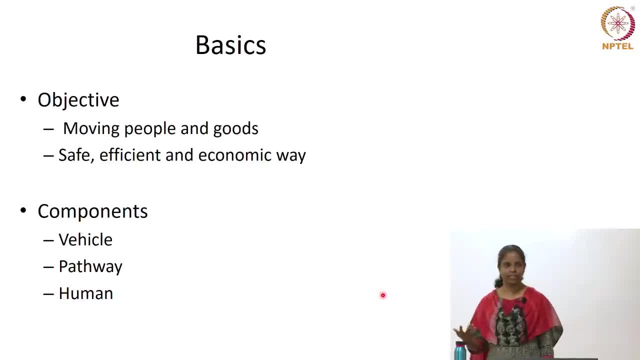 all those things. The second is the moving objects: the vehicle, the trails, air travel. So that is where I am going to concentrate maximum in this discussion, because the infrastructure is something which you are not sure of, So you are not even sure of the possible opportunities. 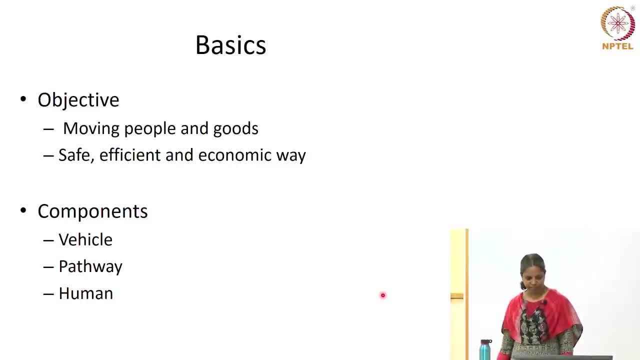 something which you already have listened to in two different talks. And the third component, which is the most complex one, is the human component. in it, There is always a driver, there is always a pedestrian who is involved in the system, and that component is not under your control. 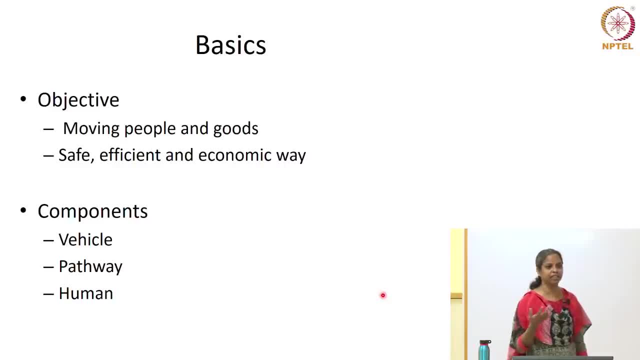 In the sense, it is not easy to model it into your equations or anything, because human behavior is very complex, right? So the challenge in terms of modeling this traffic movement, once the infrastructure is there, the most complex part, is how do we characterize the driver behavior? 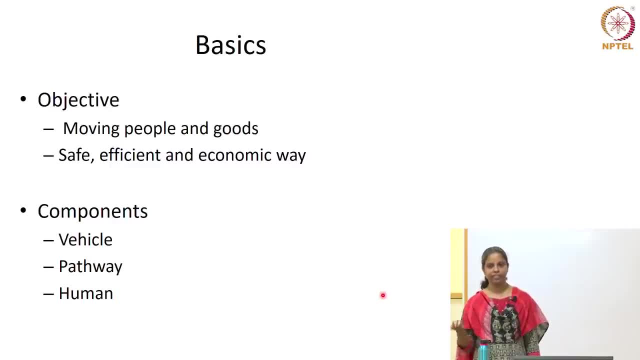 For example, different people will behave differently for the same situation, right? So how many of you have driving license? You have not used that Two wheeler at least. Two wheeler at least you have right. So you and your friend drive. 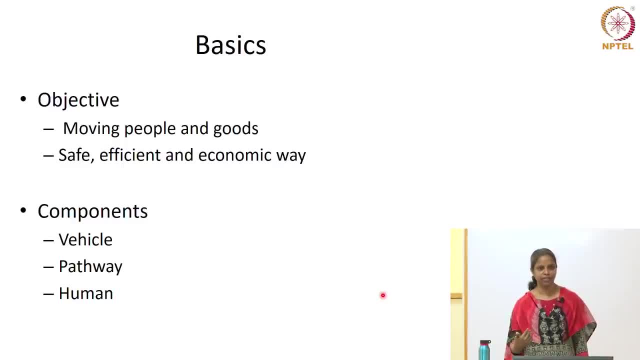 at the same time. The problem is you do not behave the same way when you have the same situation in front of you. You yourself may not behave the same way for the same situation at different time period. So if you have to kind of capture this behavior into your models, it becomes: 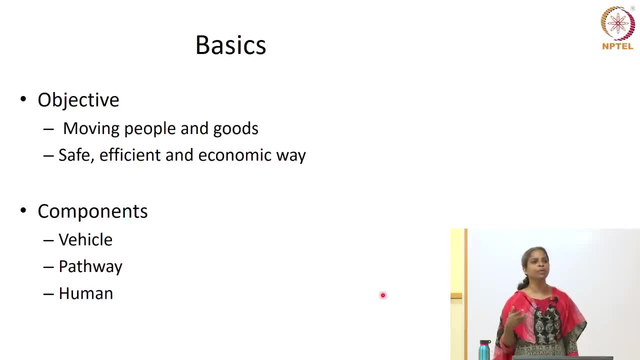 highly complex, right? So, these three components, each of those, how do we handle it? For the other part, vehicles, if you take, even if you restrict to the road, roadway movement, there are bullock carts, there are two wheelers, there are auto rickshaws up to truck. How do we kind of incorporate all? 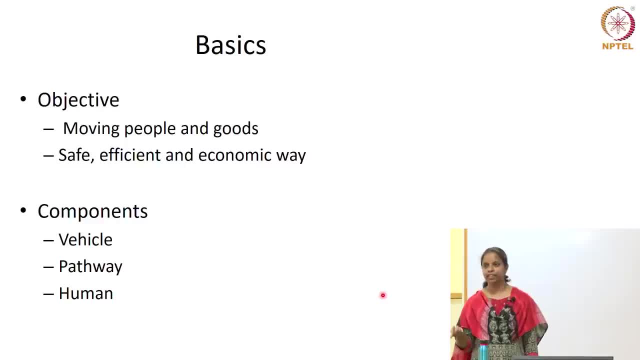 those different types of vehicles into the design right for management. How will we do that? So, and what you need is finally a system which is as uniform as possible. right, You do not want different, or you do not see different roadway for two wheelers and different roadways for trucks. 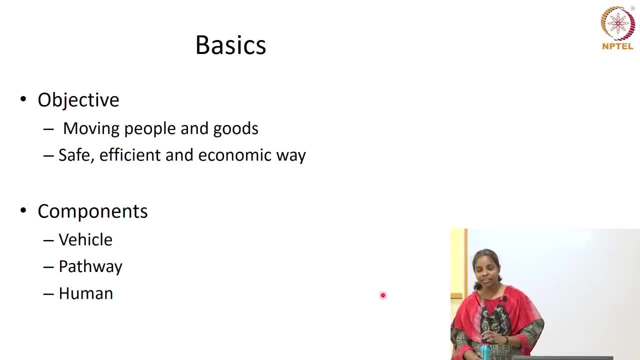 right, That is correct. The. the another challenge which you are going to see is you have varied components, in the sense you have different types of vehicles, different types of users, and you want to provide roadways and the system which is very uniform. So how do we handle these challenging problems? It is: 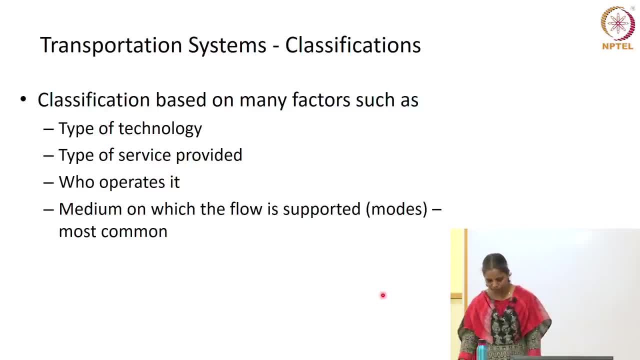 one of the problems we will talk about. So, before getting into how do we do that, what are the classifications of these systems? So you classify this system based on what technology you use, what service you provide, who operates it, what are all the? 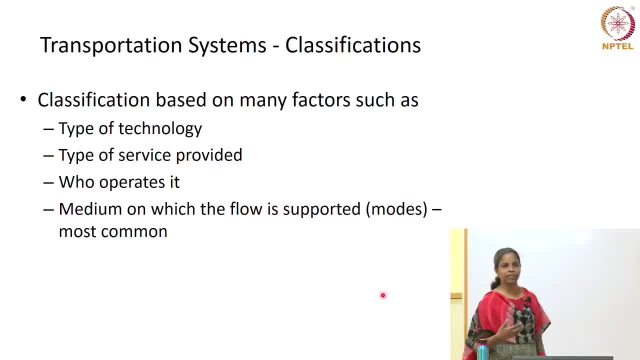 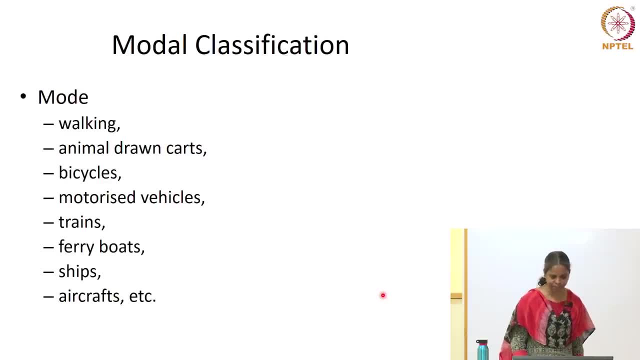 mediums. So each of these. do you understand when I say what mode, for example, is it rail versus air versus roadway, for example? that is one of the ways. So, by mode, you can see, these are all the different ways in which one can commute from one place to the other, simplest being walking. 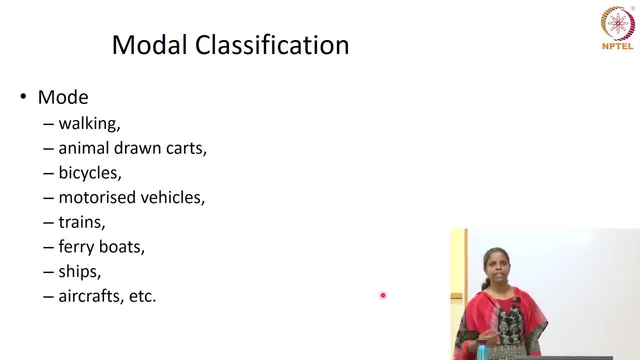 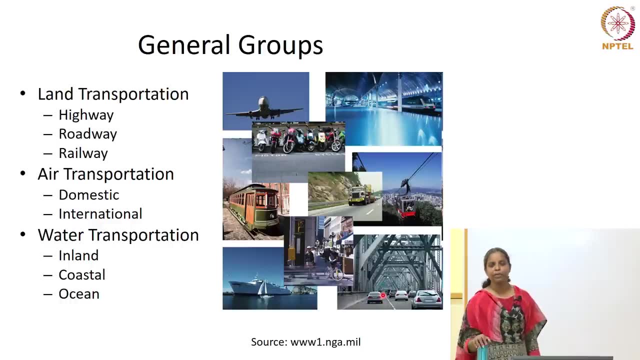 running whatever you want to. Then there are different types of vehicles. you can roadways vehicles, then there are boats, ships, aircraft, all those So in in some way. if you group this, you can say there are land transportation, air transportation and water transportation. Each. 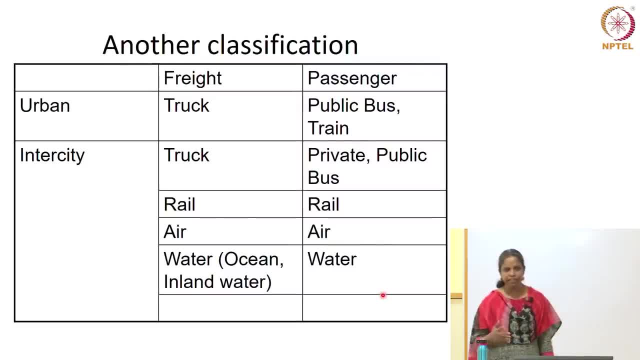 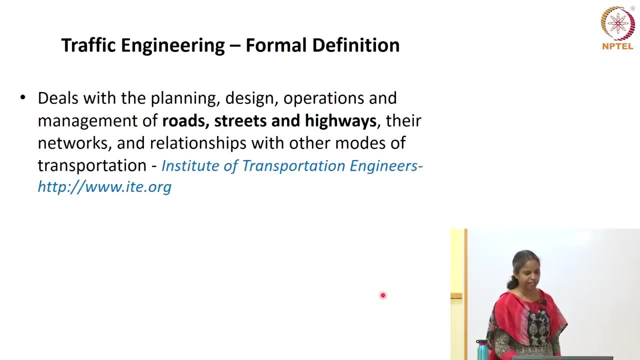 of those have a bunch of different types of vehicles. A different way of looking at the classification is urban versus, you know, intercity travel, freight versus passenger movement. How? so? each of these has uniquely different ways of handling. So these are all different ways of. 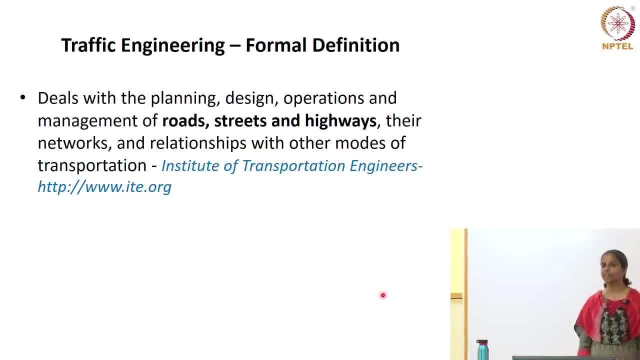 classifying the system. Now, coming to the formal definition of traffic engineering, what we saw was a very simple, crude way of starting saying that you know, move people and goods from one place to another. Here is the definition you will see in any textbook. 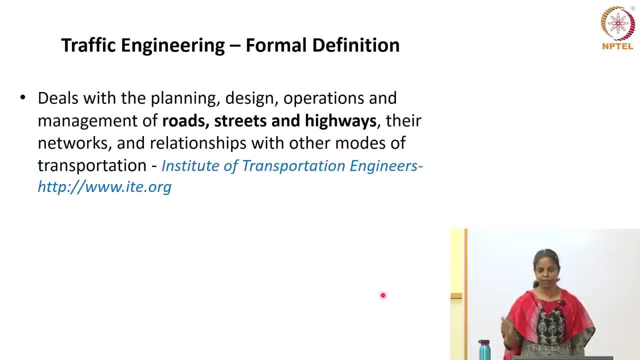 for example- and this is restricting it to the road, roadways alone- It says it is planning, design, operation and management. What he repeated is what the formal definition is. So these are the formal definitions. So these are the formal definitions. So these are the. 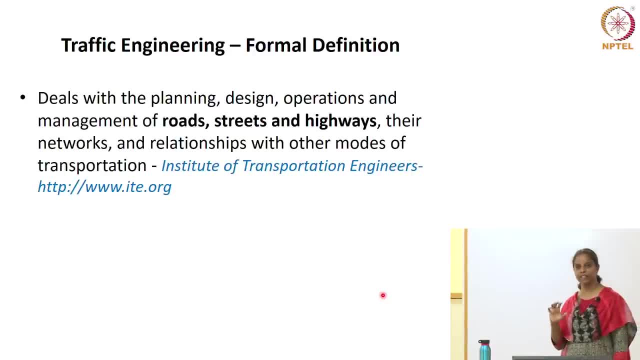 stages you will go through when you have to do a complete design or complete system development for transportation. And each of these terms- planning, design, operations, management- I will explain in one one slide. Each of this is a separate course. eventually, You have two undergrad. 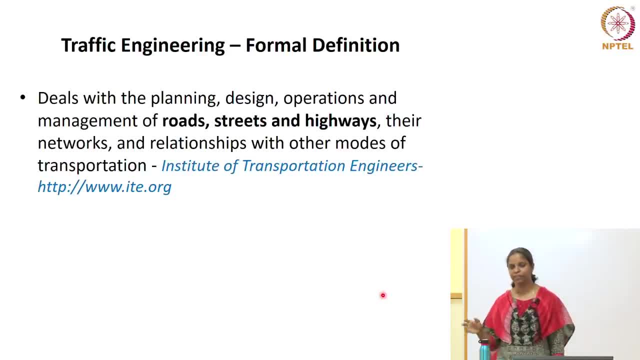 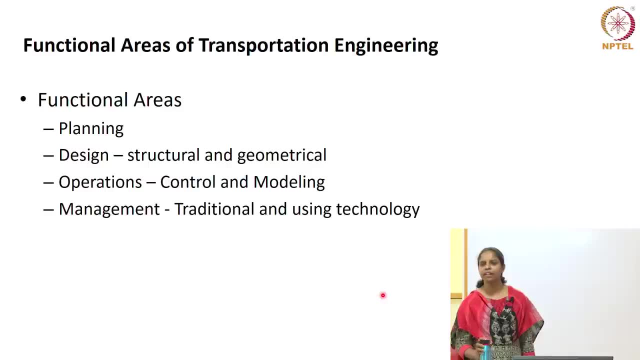 level transportation courses which will cover all these in a very brief way. Then there are separate courses for each of these, which will cover the complete details. So what planning, what design, what operations and what management? Design is what you heard little bit already from. 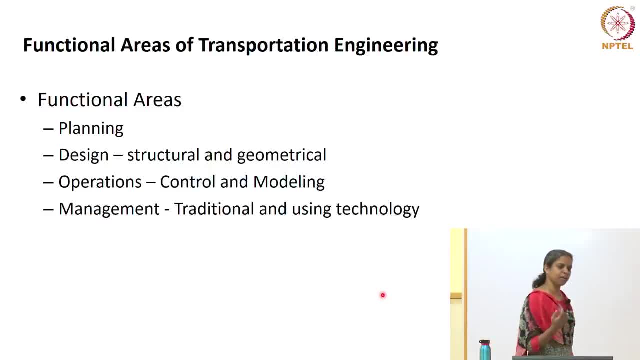 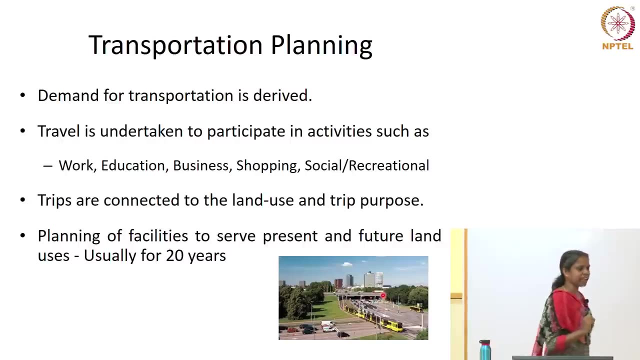 the other lectures I believe It is talked about how do you design the permit, for example, If there is a traffic known, how do you design the roadways? But even before designing you have to plan the system. So why is it important? One characteristic of this transportation is you do not usually you. 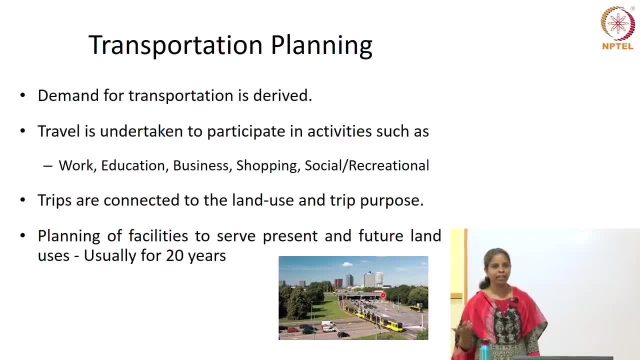 do not always plan the system, So you do not always have a plan of what the roadway will be, what the traffic, what the roads will be, what the roads will be, what the roads will be, what the Usually you don't make a trip just for the sake of it. 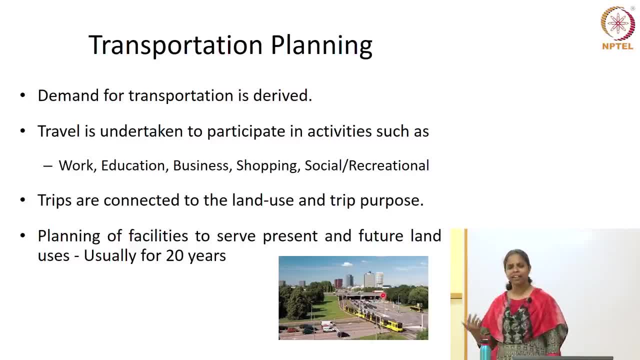 You don't go for a drive- Okay, very rarely. maybe one person you will be just for the thrill of riding a bike or something. you will be there, But most of the time you are traveling for some other purpose. Either you are going to your class or you are going to a movie, you are going to visit someone. 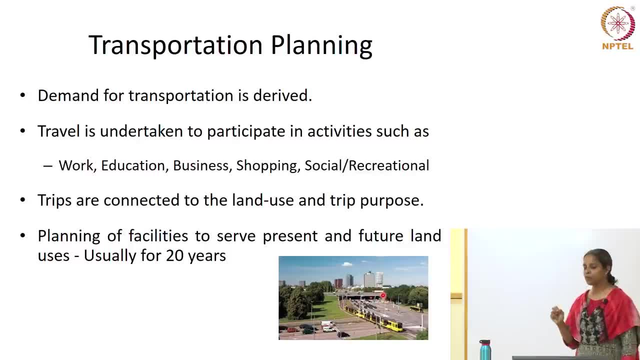 So there is an end reason for you to make the trip. So that's what is meant by the derived. There is a term called it's a derived demand. So the trip you make is related to some other activities. Most of the time it will be socio-economic related thing. 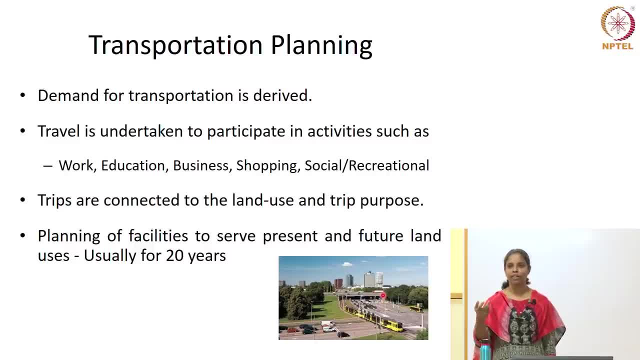 So the land use plays a major role in what trips happen. Correct? If it's a recreational area, the trips are mostly to visit the place. If it's a residential area, the trips are usually people want to go to their workplace or they want to go to their colleges. 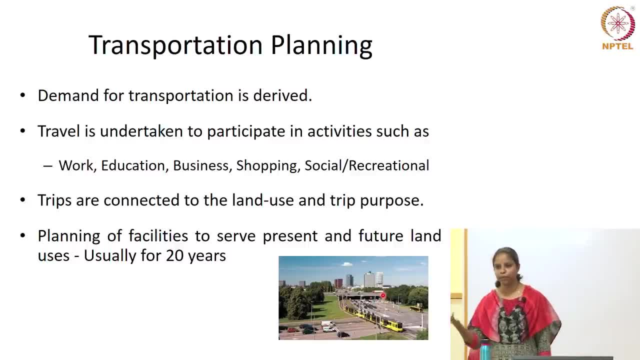 If it's a shopping area, people go for shopping obviously. So each of these trips is related to the land use of that area. So the planning part kind of leads the land use to the trips that you make. So when you say you want to plan something, or when you want to plan transportation system, 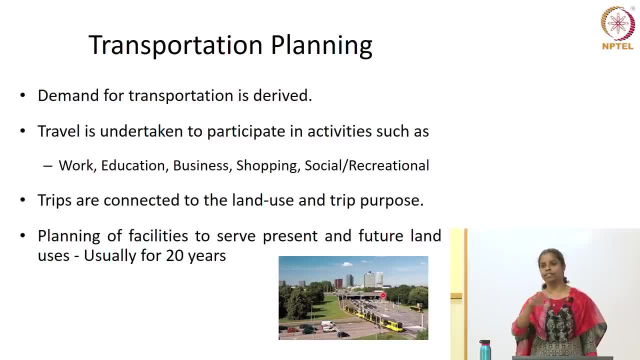 you start with the land use of the area. So if, let's say, somebody says that they want to move the capital from Chennai to some other city, So you will have to design the entire transportation system there. So you will start with looking at different zones in that area. 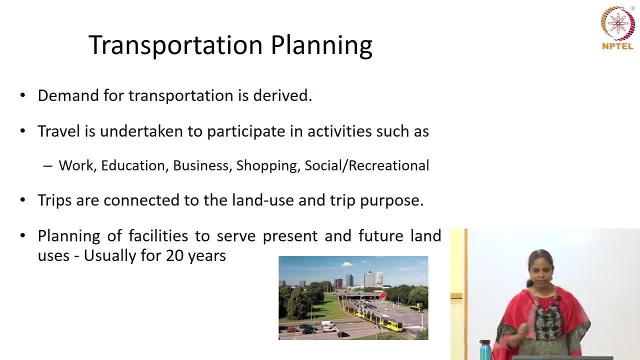 what is the land use of each of that area. then you start planning. So how do we do that? And usually this planning and design is done for a period of around 20 years- 15 to 20 years. So the planning part has four major steps. 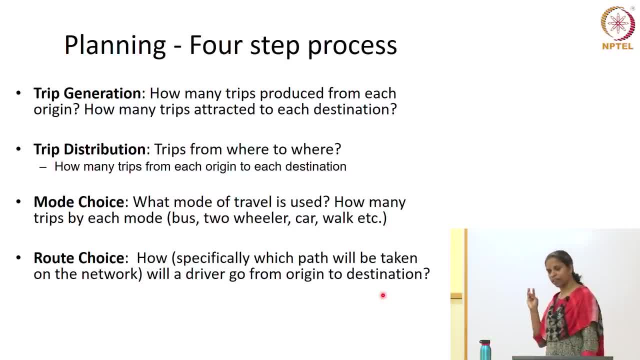 I am not going to get into the details, But it's. they are called trip generation, trip distribution, model split and route choice. So what we are saying is: first, you want to find out how many trips are generated from each place. 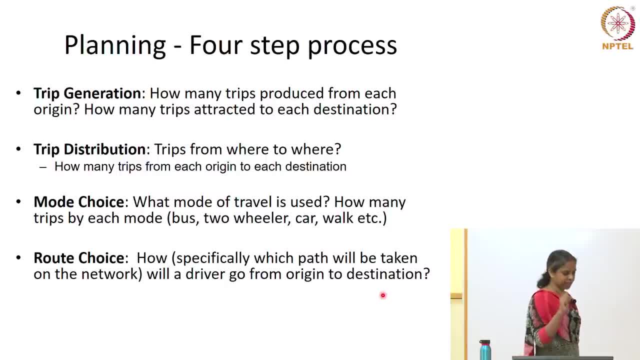 or how many trips are attracted to each place. in the first step, first stage, Second stage, what you are doing is you are trying to say: from this zone to this zone, this many trips happen. That's the trip distribution step. 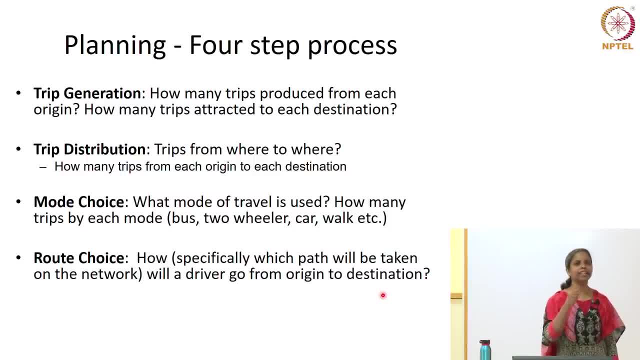 Then you are looking at how many of those trips are done in different modes: two wheelers, how many cars, how many public transport, how many, And the last part is which route each of these trips happen. So at the end of this fourth stage, you know from each zone to each zone. 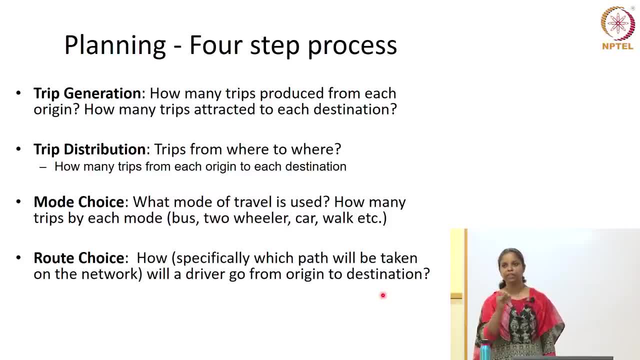 how many trips happen by each mode through which route you understand. So at the end of this, you know that this route, this many two wheelers and this many cars have to go. Then you get into the design, where you will use this information to design what type 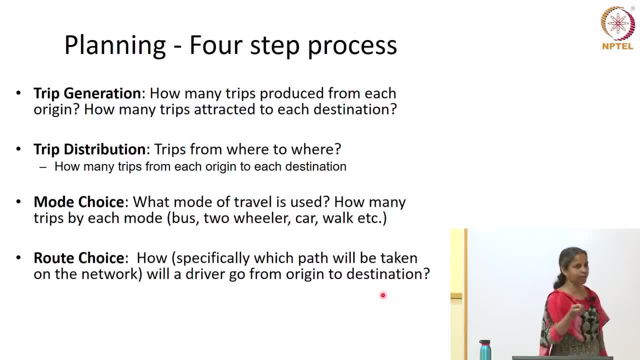 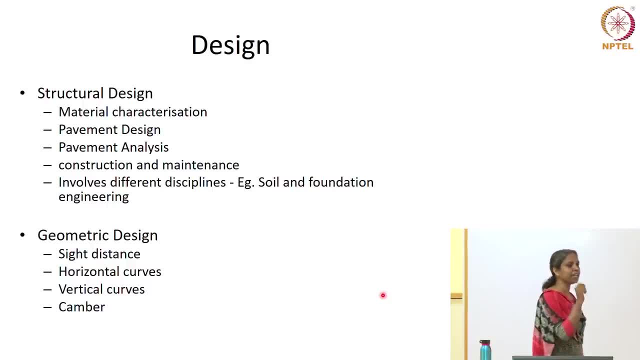 of roadway. you need, how much thickness you should do, what material you should use, and all those. So that's the next stage, which is the design. So there you are looking at how do I define this system for the roadway. 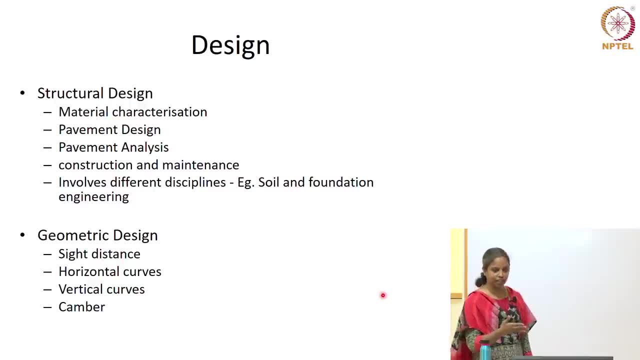 So you will be getting into what I said as the hard side of it. basically, you are looking at how do I do the Okay, Got it of the material, how do I design the thickness, how do I check the structure and frame. so 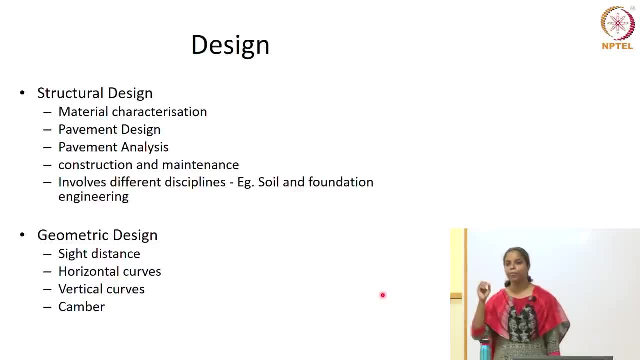 that is generated, whether it is safe, whether it will crack all those information you need. So this is more of the structural design of the roadway. That is one part. You would have heard some lectures on structural design of buildings, Similar to that. you are talking about structural design of roadways. 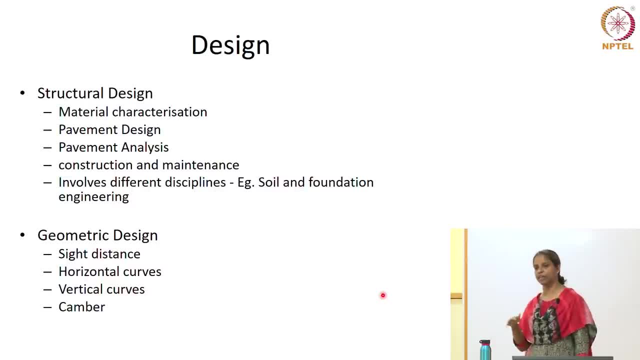 Once that part is done, the other part is the geometric design, where you are looking at how do I design the curves, how do I make sure that the vehicles are not thrown out when you are negotiating a curve, or how do I make sure that a vehicle does not slip back? 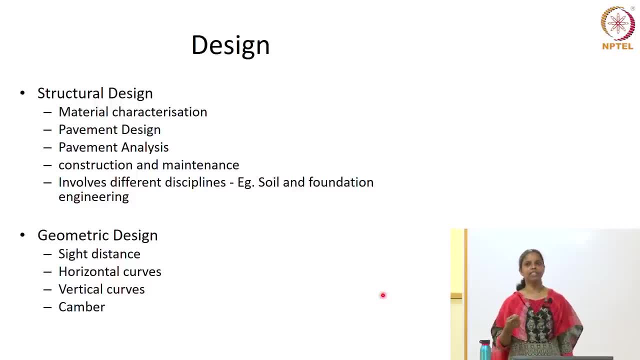 when they are climbing an uphill. So you have to make sure it is done correctly. So that is the geometric design part of it. As I said, each of this is a separate course. Geometric design of highways is one separate course and is offered from the transportation. 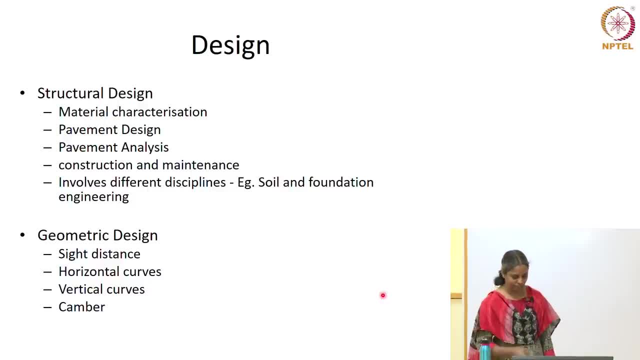 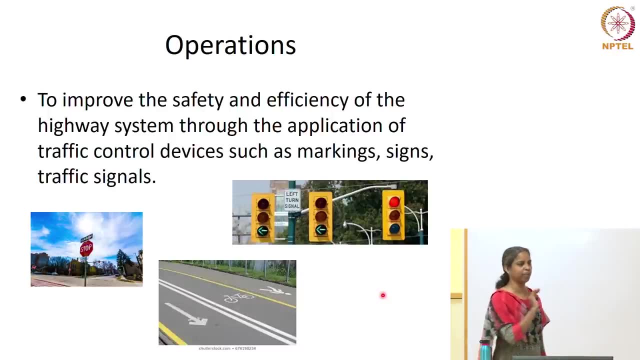 unit. So this is the second stage. So it was planning design. Third is what is called as the operation. How do we control or manage the vehicular movement on a roadway? So there is no way you can communicate with the driver. 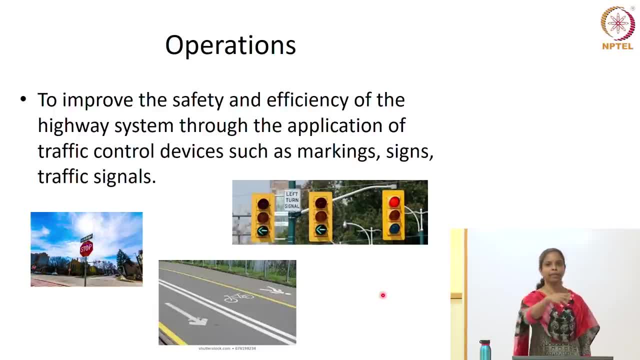 As an engineer, you do not communicate with the driver by calling hey, you cannot go this way, So you need some kind of media to communicate with your driver. That is what this operations mainly is. It is mostly about signs, markings and signals. 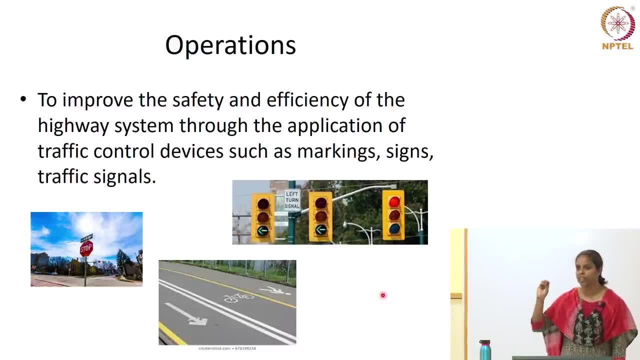 You would have seen all of this. So markings are on the roadway, signboard sit in the roadside, and then signals sit there, either in the roadside or across the road. So these three kind of tell you how you should behave in a roadway. 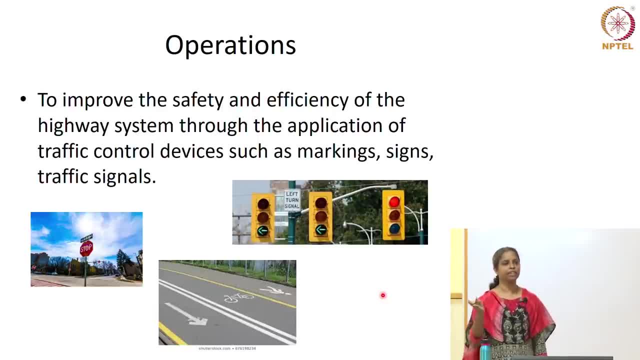 So the operations usually is: how do you design the signals, how do you make sure the signs are correctly placed and correctly conveying the information that it should be? So it is again separate course which is on signal design, signal analysis and all those. 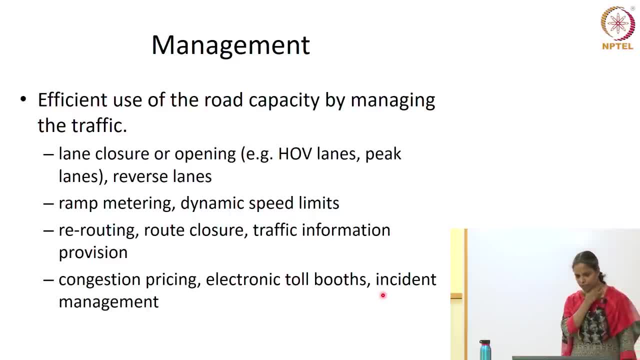 things. The last part is most important, So the operation is basically on the management. Once you have this, how do we handle the traffic? still, you know, in terms of mostly you see this being done in India by the traffic police, right, 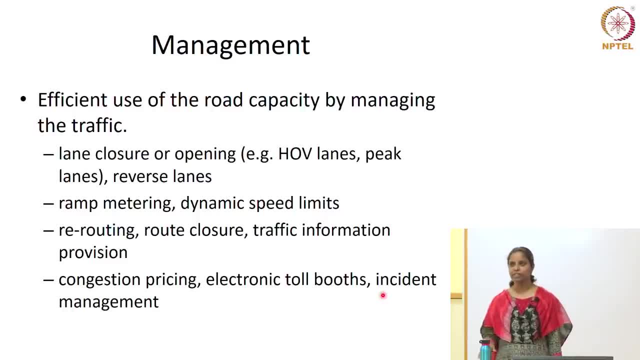 Suddenly the traffic police decides that this road has to be a one way because there is there is problem. Ideally it should be done by traffic engineers, but here mostly the police people do that. but these are different ways in which one can manage the traffic. 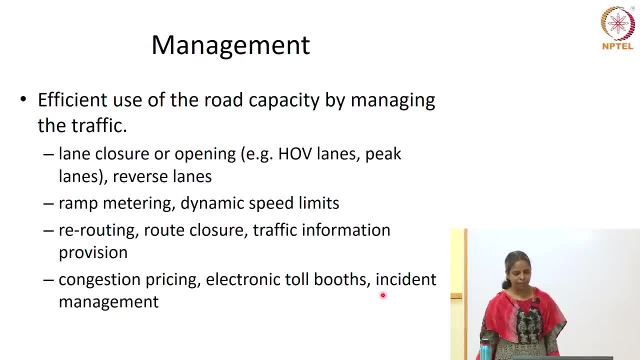 Once you have the roadway done, signals sit there, There is information in place and all ok. So, having said these four steps- planning, design, operations and management- we will mostly concentrate on the operations and management part. That is what the soft traffic side of it. 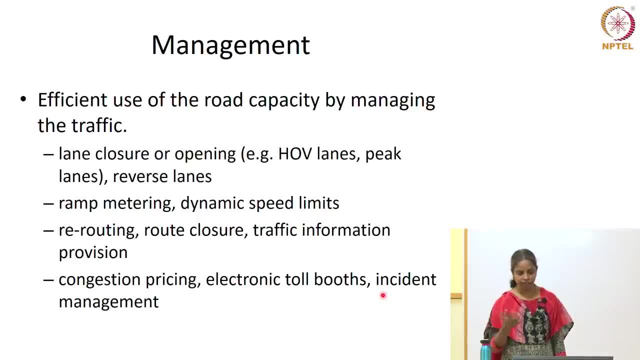 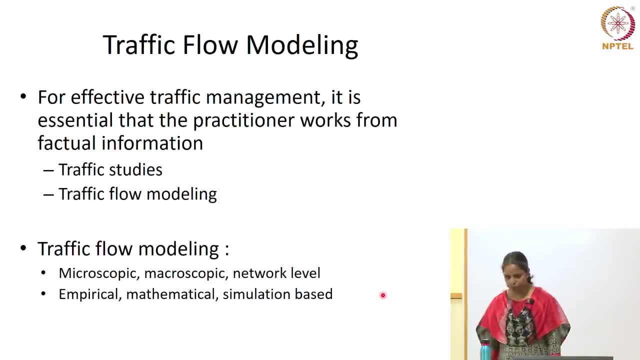 So you have the planning done, signal design, a sorry roadway design done, and how do we make sure they are moving efficiently? right, That is what this is. So one major part is you have to model the traffic. Yeah, Yeah, Yeah. 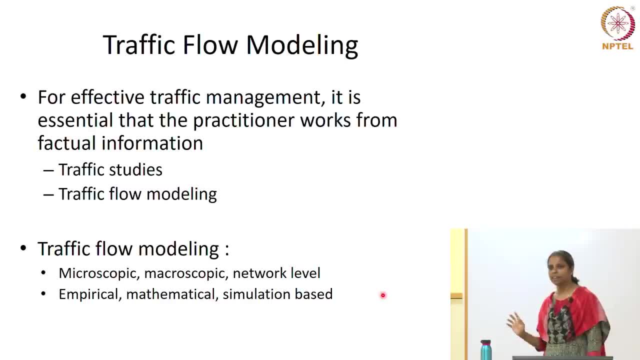 Yeah, Yeah, Yeah, You have to kind of. you have seen, you know, modeling of different things, for example, rocket. if you have to design first, you start with equations that will design and decide how it is going to move, how it is. you know trajectory is going to be also. 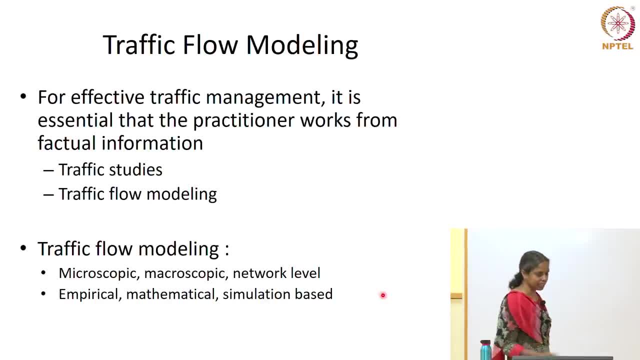 Similar way, you have to have models which will characterize how this traffic is moving. It is, in one way, to find out how this traffic is going to behave at different time and different location. that is what the modeling is trying to do, And for doing that you have to collect lot of information. traffic studies will come. 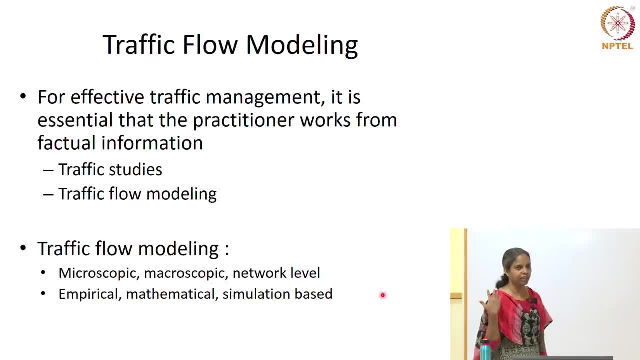 up and then the modeling part, which can be statistical modeling, it can be mathematical modeling, it can be just data driven models, empirical models, all those, but some way you want to model. And the other question is: how do we model this system? there are vehicles, then there. 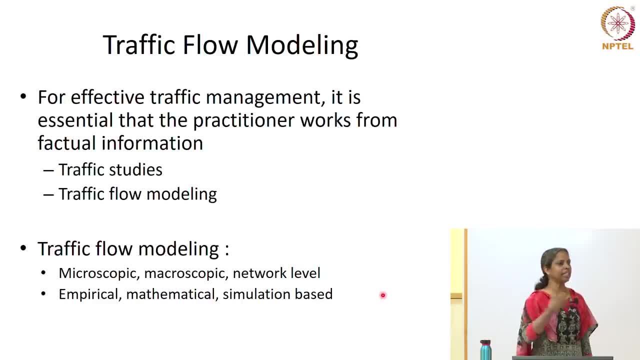 is all the vehicles moving on the roadway, then there is the city level network, then there is the traffic. So which one you do you model? that is where these terminologies come. there are microscopic models, which are individual vehicles. how do they move? 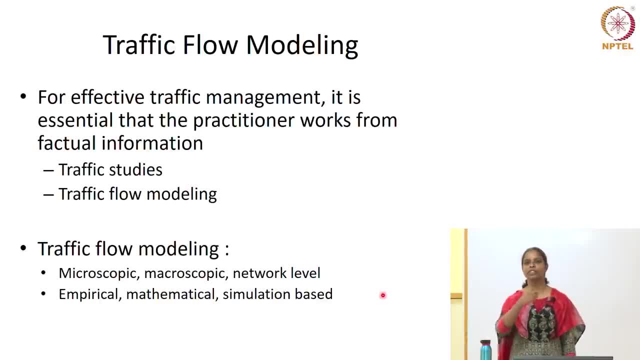 The macroscopic models kind of come out with equations or ways in which you will know how the traffic as a whole is moving. Then there is network level, in a city level. if you want to model- you do not do even at every road- such how the traffic is moving. 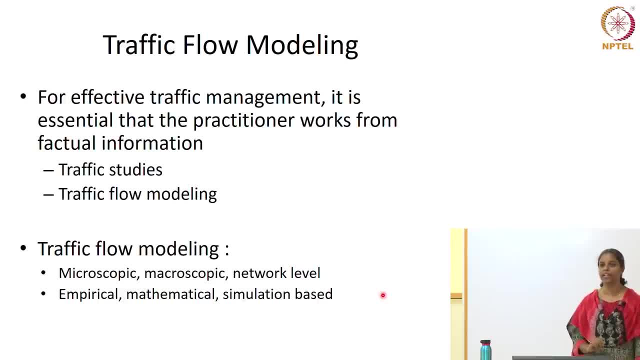 So how do we do it at the network level? It is challenging in its own way because, for example, if you take microscopic level, how one vehicle will follow its leader. it is challenging because it heavily depends on the human behavior, the driver who is sitting in the vehicle. 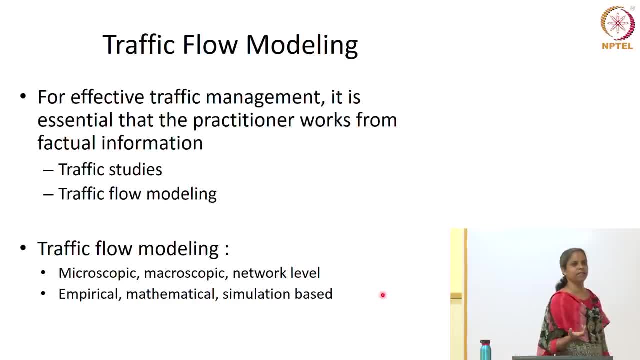 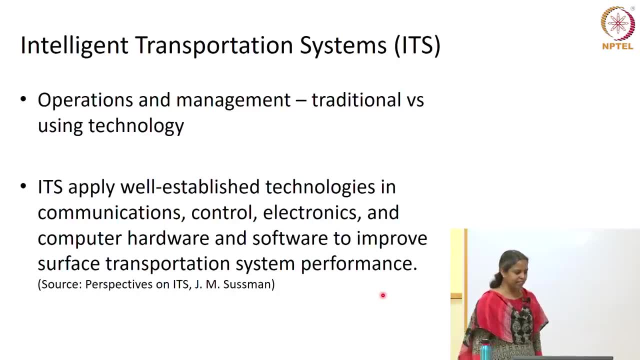 So how do we include all these into the modeling and have some reasonably good models is what comes under the discussion in traffic flow modeling, And this is something which is more recent. by recent I mean in 70s. it started, but still. 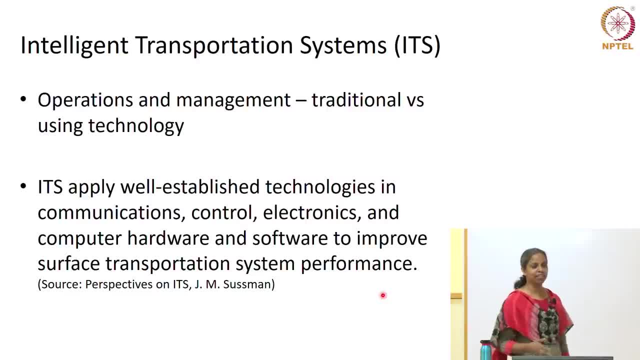 the other things are coming. Ok. So in the 1930s or 30s, so 1930s, this is, in 1970s- what called as intelligent transportation systems- Many of you would have heard this term, I hope. 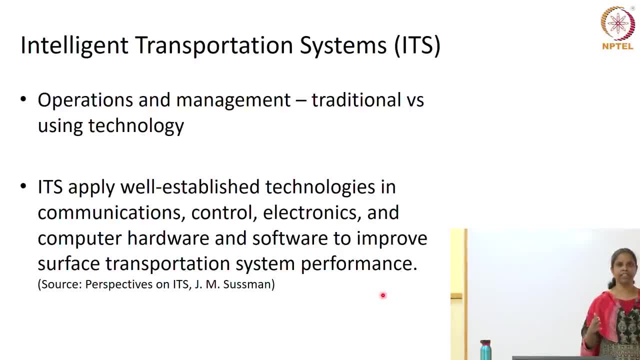 So what we are talking about is, so far, whatever we talk was done in a very traditional way. you know, you collect some data by going there manually collecting, analyze it, come out with something With latest technologies in terms of sensors, in terms of communication, in terms of analysis. 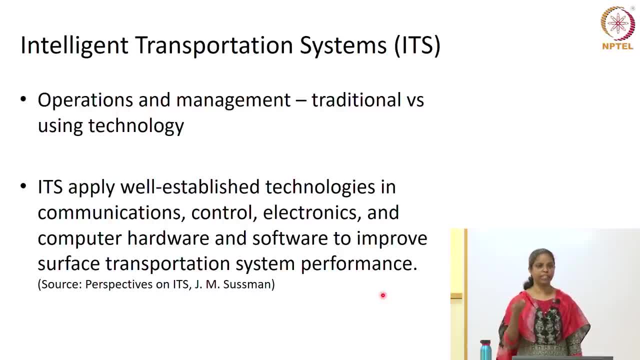 there are new ways in which you can handle these problems, whether its operations or whether its management. So that is what the intelligent transportation system is. So this is again a textbook definition. it says that any advance communications, control, electronic, computer related technologies being used in traffic. 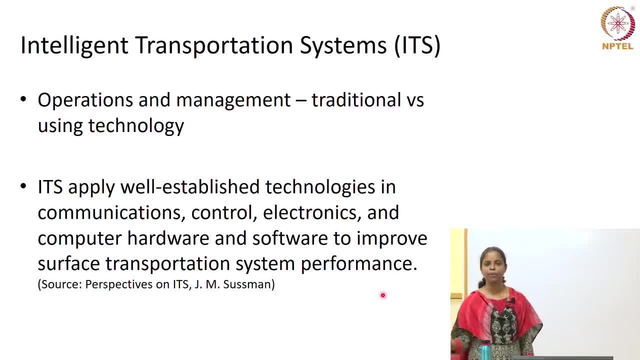 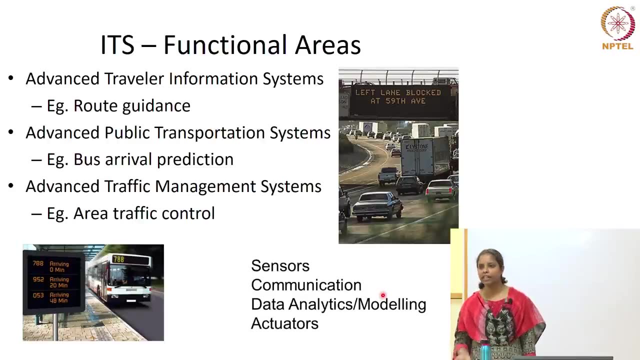 That is what the intelligent transportation system is, So I will just quickly discuss a little bit on IPL. Ok, Thank you. I will just quickly talk a little bit on ITS, because the latest trends in terms of connected vehicles, automated vehicles, all those comes from this starting point of ITS. 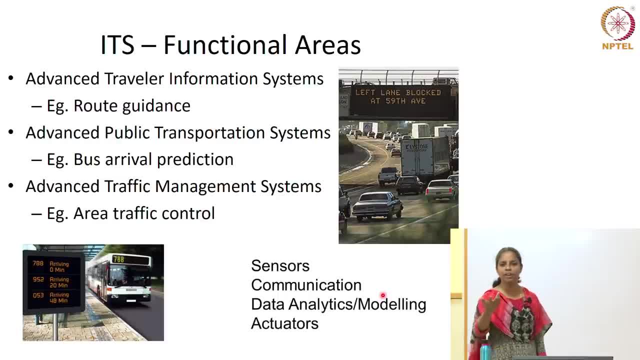 So ITS? there are many examples. your Google driver assistance is a classic example of a ITS technology. What do you get there when you are using a Google map? When you start your drive, usually you do right. whoever is driving, keep the Google map ready. 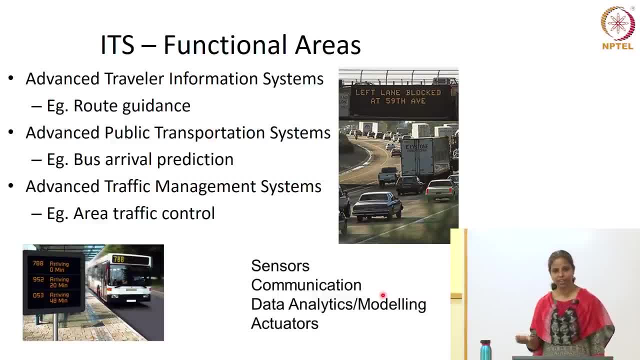 there, this is my destination, which route I should take or how much time it will take. right, How is Google coming out with that information? Any thoughts? It is ok, they are recording, but that is fine, you can talk. 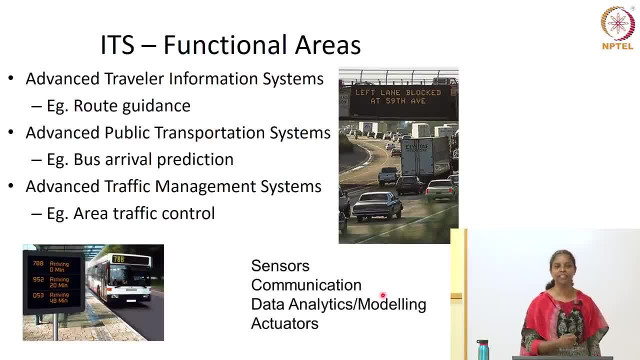 No thoughts. How is Google coming out with this information that you know this much time it will take for you to reach this point? Satellite, How will satellite get that information? Ok, it is all coming from your cell phones, ok. 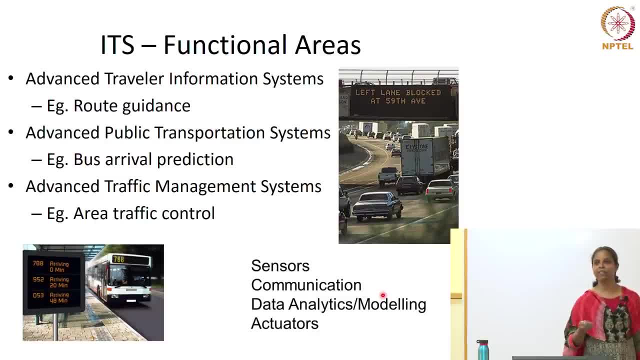 If you use your Google Maps, there will be some fine print somewhere there that your data will be used and many of you are using it. so they know roughly what is the traffic situation in that road at that time And they have their own analytics in the background to calculate and tell you: ok, this is roughly. 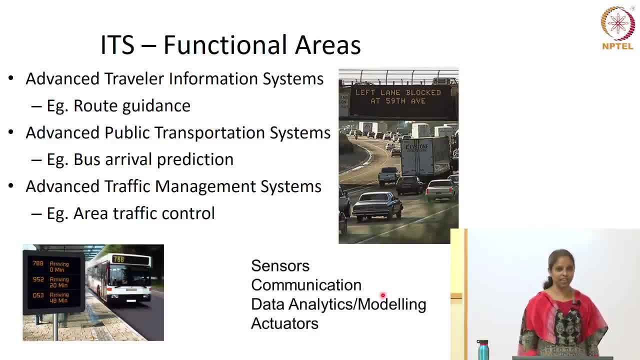 the time it will take and this may be the best route to take at this point. Right, so there are many examples that you can. you have seen already, For example, route guidance. Google is one example. Pictures like or message boards like this: it will tell you which route to take, how much. 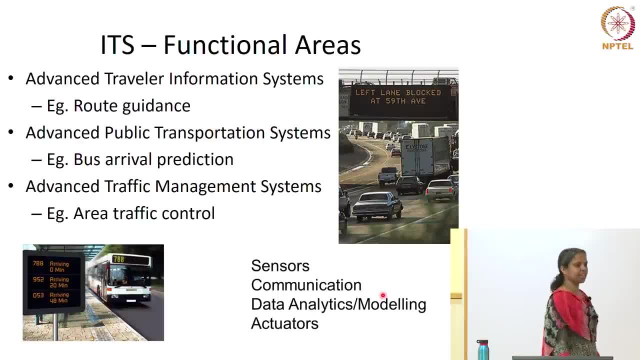 time it will take, Or bus arrival prediction area traffic control signals being advanced. The current signals which you see, for example, have static time. it always have this much time of green, this much time of yellow and this much time of red. 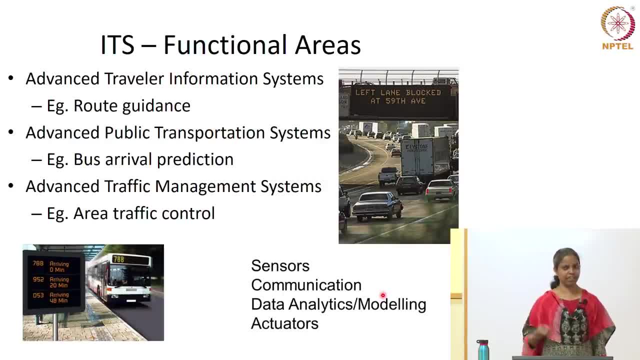 And there are times in which you go there, you are in a red, the other side is not having any vehicle, but they have a green Right. It is kind of frustrating. So how do you make it advance If you, if there is a way to collect the information from each of those legs and process it, and 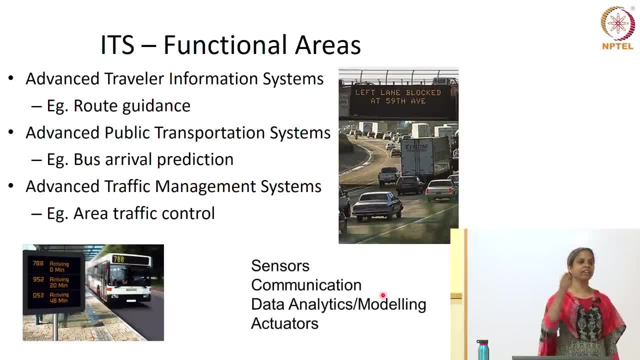 tell: ok, this leg, there is no vehicle, so do not give any green. this leg has vehicles waiting, give green. So if it can happen in real time, that is an example of IT. So what did it do? 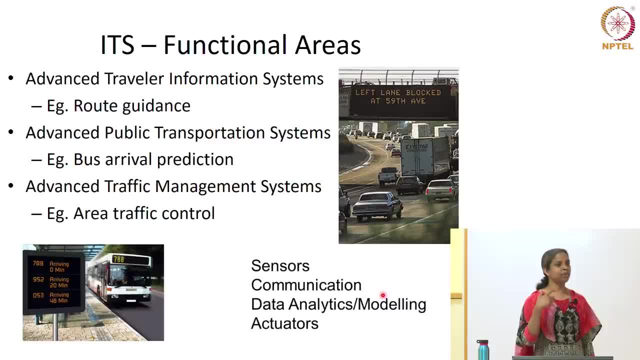 It collected the real time data, processed, it found out what is the best, So it has a way to handle it and then change the signal accordingly. That is a classic example of a ITS application. So if you look at any ITS implementation, the four major components is sensing the data. 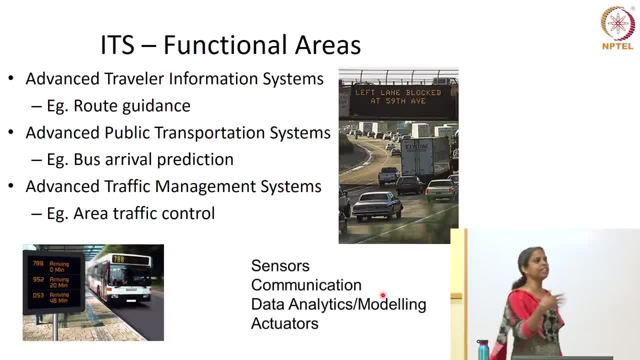 communicating the information, processing the information and then deciding what to do. or, you know, actuators which we kind of give back this information to you. So this needs lot of sensors. obviously, Right, The sensors can go into the vehicle. the vehicle can go into the vehicle, the vehicle can. 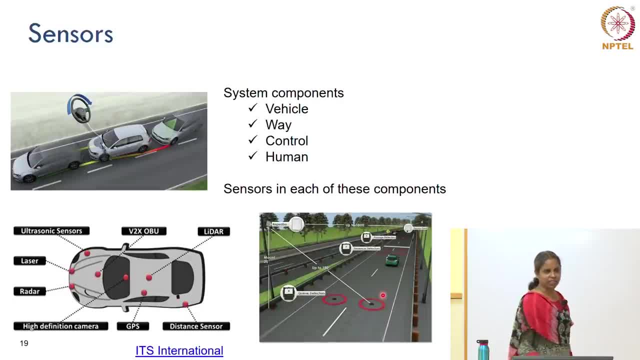 go into the vehicle to get information. So this is the main component. What is the central structure? This is the central structure. So this is the central structure. So this is the central structure. be at different places: it can be in the vehicles, it can be in the roadway, it can be in the 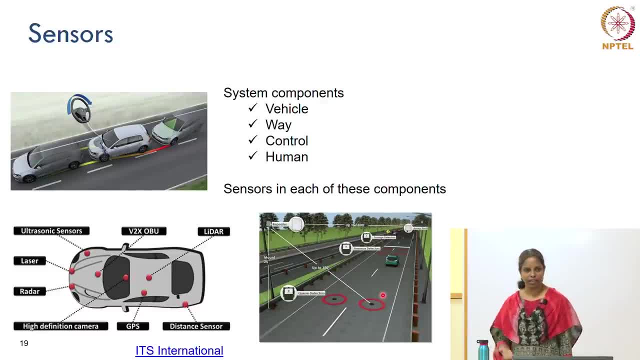 human being. So, and with the advancements that is happening, there are enough sensors. that gets deployed into your vehicles for definitely there within you. for example, your cell phone is a very good sensor. it gives lot of information. then, road side, there can be enough sensors. 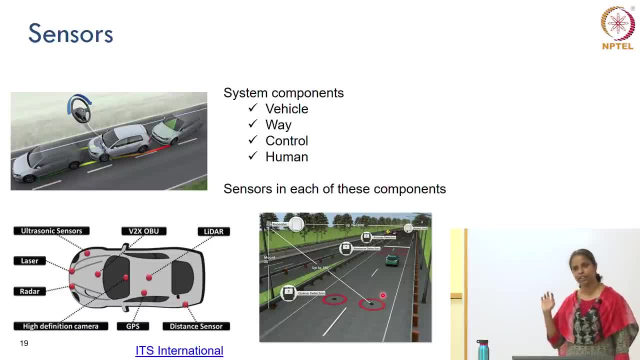 Slowly, we are also reaching there. many other countries already have sensors deployed everywhere, and all these sensors are communicating with each other, which leads to what are called as V2X communication- internet of things. you must be hearing all these terms right? So every device or every component of the system is now giving information to each other. 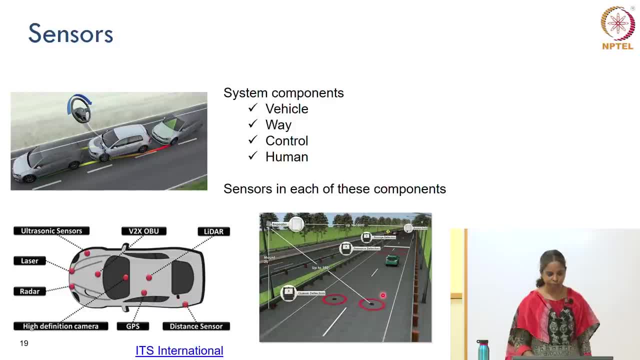 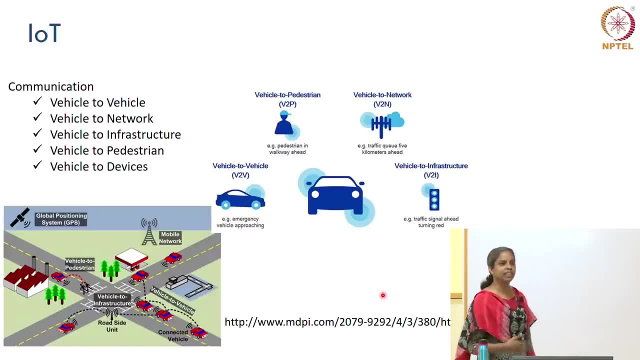 they can process this information and know how the traffic is moving. So these are different systems. These are ways in which you can have sensors in a vehicle or road side. So, as I said, this leads to what are called as internet of things. communication can be. 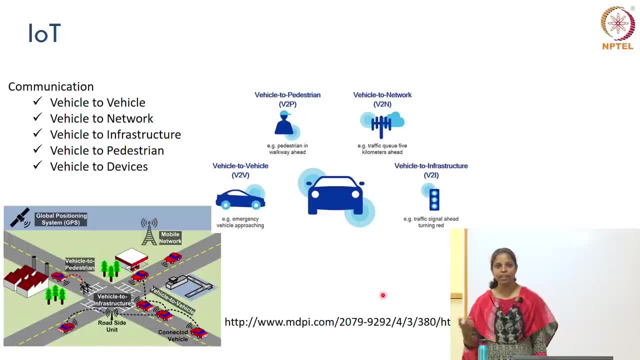 vehicle to vehicle, V2V, V2I, V2P, So in general, V2X, vehicle to anything. communication can happen And this is the basic component or basic concept from which this connected vehicles. this is one of the hot topic you will hear connected vehicles. 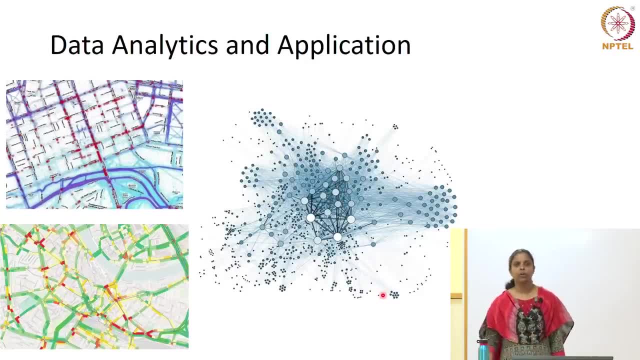 That happens because of all these things. So these are all these information and, yes, once you have lot of sensors, lot of data, So you have to get into data analytics, So a lot of information can be processed. If you ask me, I am still somebody who believes you know. back to mathematical modeling is 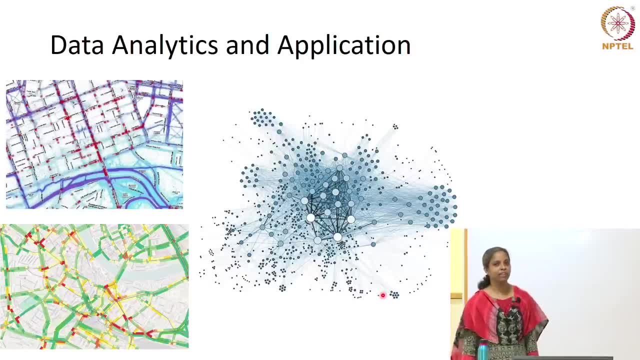 best, but I am getting to want to be wrong. There are places where lot of data actually gives you enough information than a mathematical equation can capture, So there are cases where data can be processed. There are cases where data can be processed. 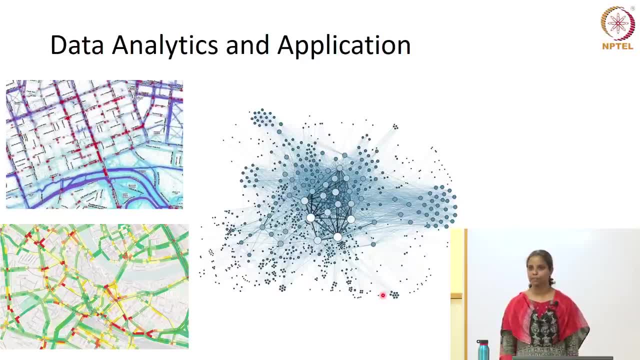 So there are places where lot of data is available. it can make sense. So there are, at least you know. Google and all are using data analytics today. They have lot of information with them. They have just process. They do not try to understand the physics of the problem. 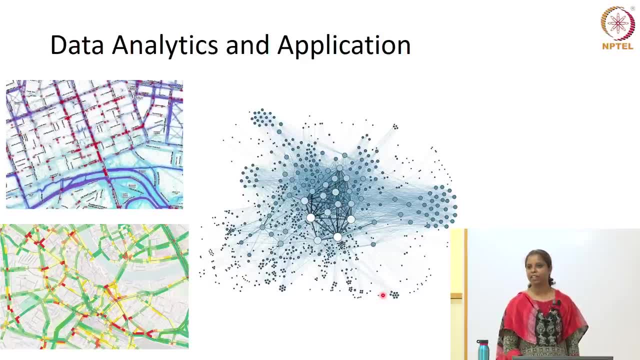 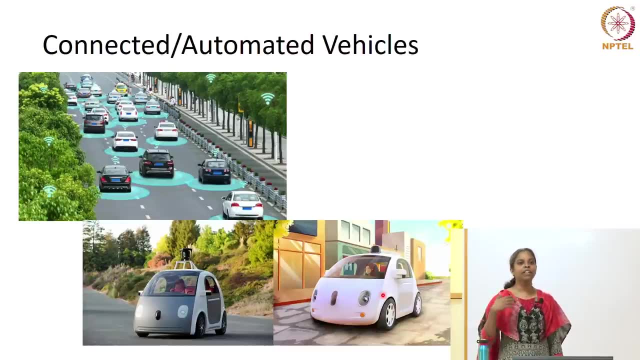 They just look at the data and the behavior and the pattern so that they will they will be able to give you information. So, as I said, this leads to what are called as the connected vehicles and automated vehicles. You must have read about this: Google's driverless. that is the way the data is calculated. 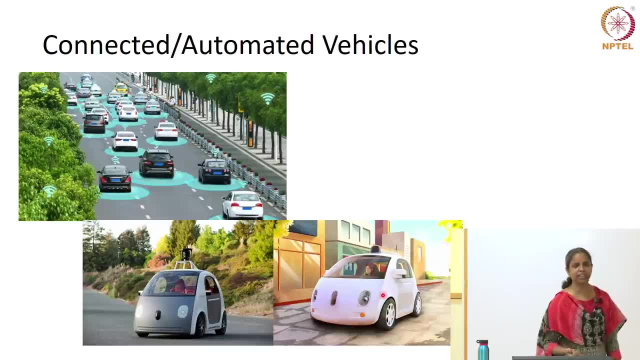 driverless cars and all those things. there are enough countries where they are already running in the roads. Will it come to India? It needs time, needs lot of time, because we have a very unique way of driving, but in many other countries we have these kinds of vehicles. 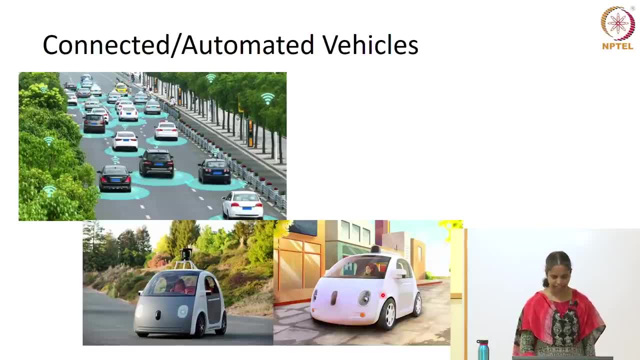 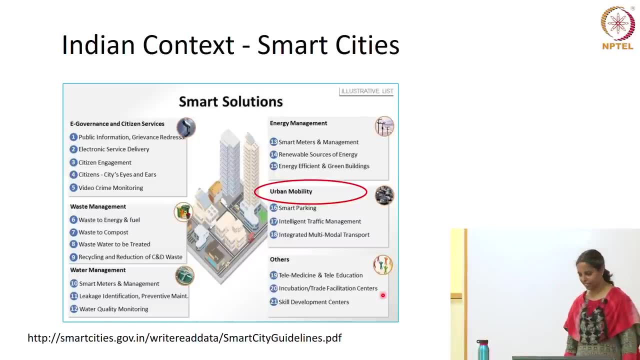 So all these, the starting point is having enough sensors and enough communication happening. That was kind of quickly giving you an overview of various things that can come up from this traffic engineering and planning side. Having said that, I thought I will just tell you where. what is the Indian context to all? 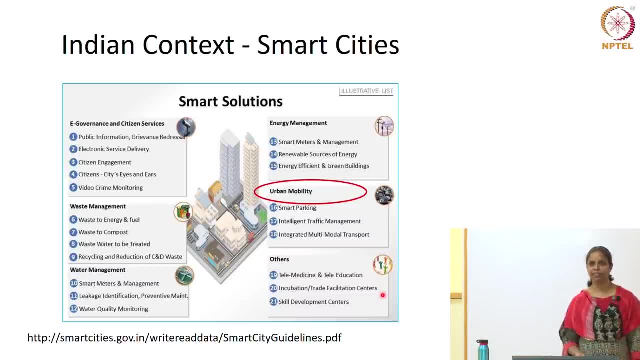 these. So some of you may be thinking: why are we talking about connected vehicles and all when we are still building infrastructure? it can happen in parallel also, So this is one way of looking at it. You, you again, would have heard about the smart city initiatives of the current government. 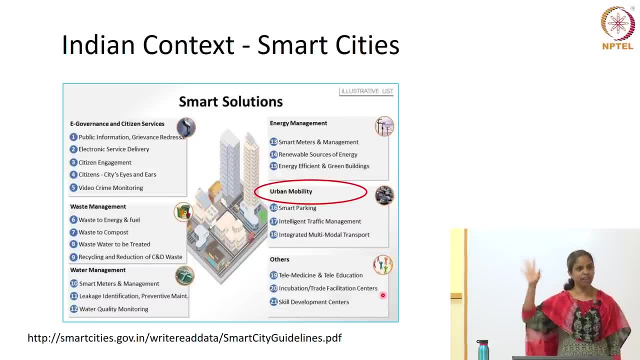 previous term itself. So mobility is one of the ways. So these are the verticals under the smart city initiatives and that is what I have highlighted. They have given some examples: smart parking and intelligent traffic management, integrated multi-model integration and things like that- but it is not the. these are all the only things. 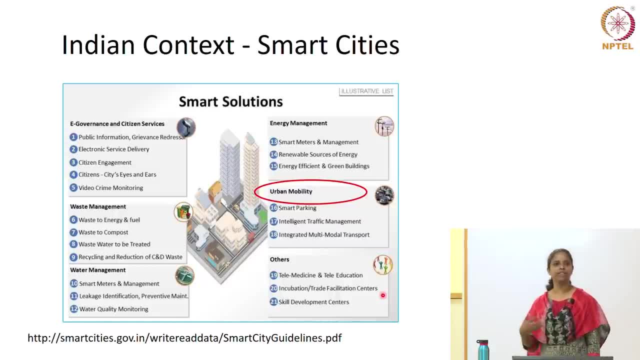 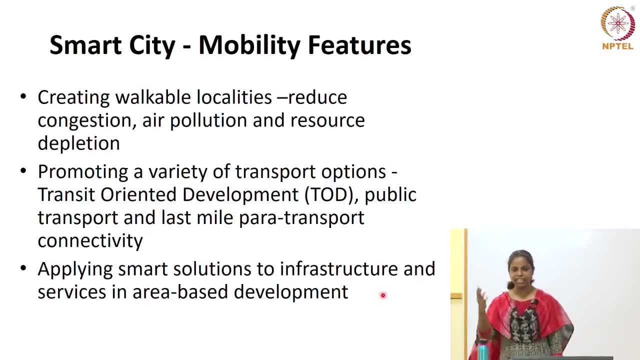 They are interested in anything where you can use technology to make the traffic move better, So that is where some of these things can make sense. These are some of the details I collected from that website, where they talk about what is a smart city. 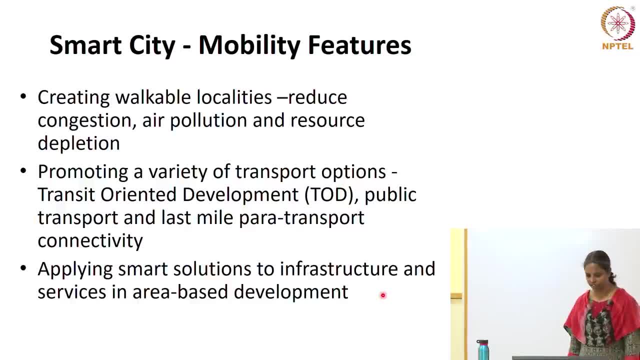 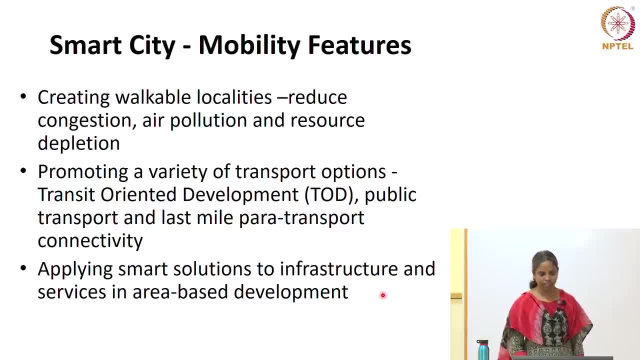 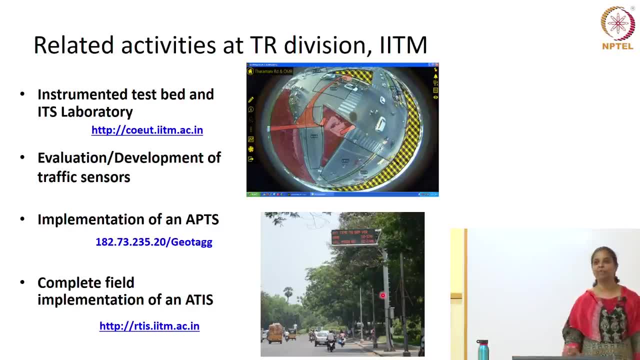 in terms of having such developments to be done- And yes, I have to do some PR work also to excite you. So these are some of the activities that that are happening in our lab related to this ITS, or traffic operations management, and all that. 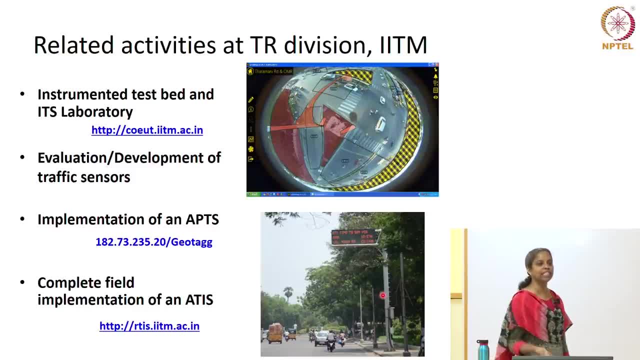 of the examples just to show what your seniors have done. many of the work which I am showing are done by undergrad students either as part of the curriculum. mostly they were interested so they just start working on it. So I have put mainly the activities are. we have developed a laboratory which is- I will 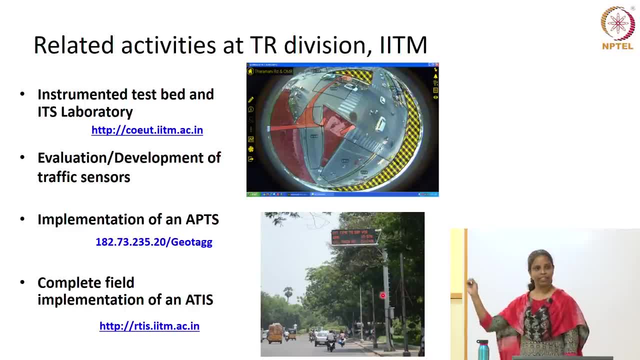 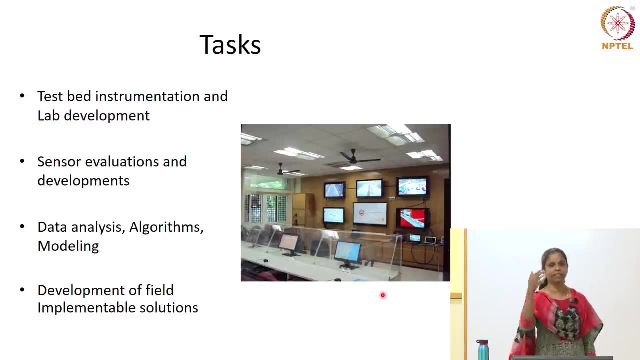 I will show you some pictures- and we have a test bed, live test bed, from where we are getting data. then we have developed lot of sensors which was for our traffic conditions, then some of the solutions we have developed and implemented. So, as I said, one of the the tasks I have divided into four headings. one is the lab development. 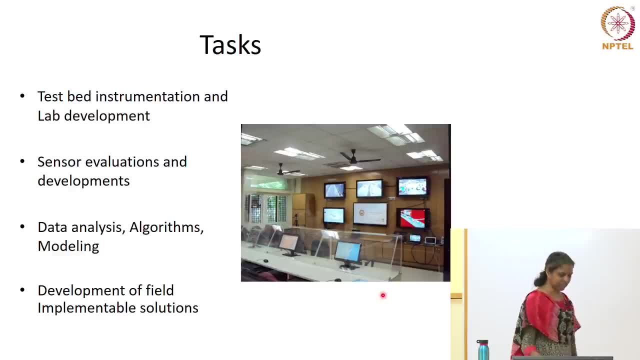 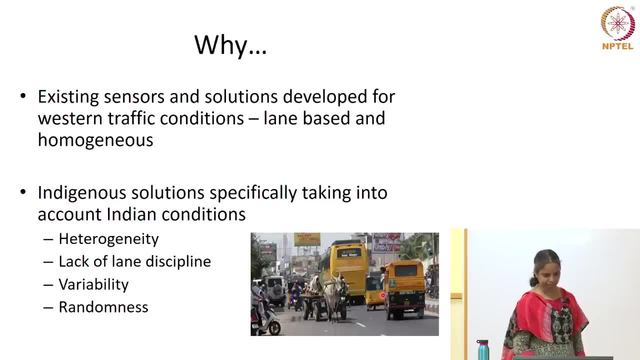 and the test bed sensors, then data analysis and the solutions that we develop. this is the picture of our lab. any of you can come and see the lab when, if you are interested, we will make sure. So before I get into the details, why do not you go ahead and see the lab? 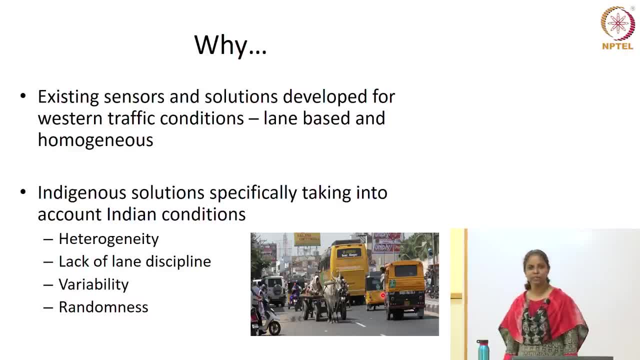 Okay, So the first thing we have to do, right? I do not think I have to explain much. you know that our traffic is completely different from what you have seen elsewhere and all the models, all the solutions that are developed are actually for the traffic which is lane based and homogenous. 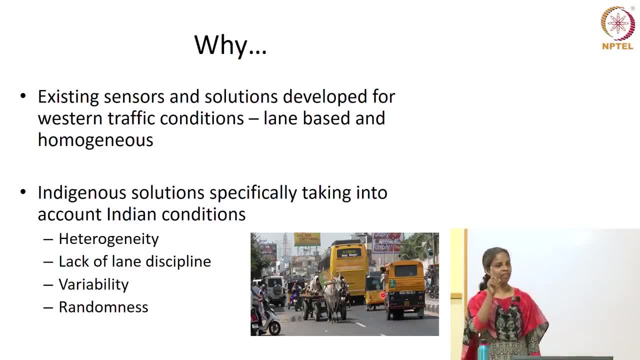 by lane based, I mean them in one lane. you expect only one vehicle. they move one after the other. they do not move parallelly within the lane, which we happily do. We do not believe in this. you know, follow the leader of behavior. we will occupy any. 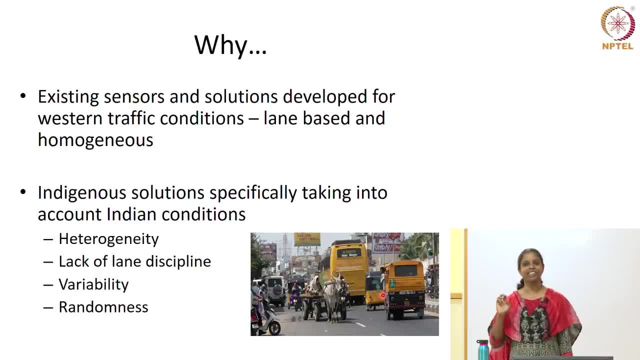 space available. So it is in one way interesting: we are using the whole available space. we do not want to waste anything. but the problem is modeling. it becomes extremely difficult because you do not know how the vehicle is going to behave. right any gap you see. a two-wheeler can move. 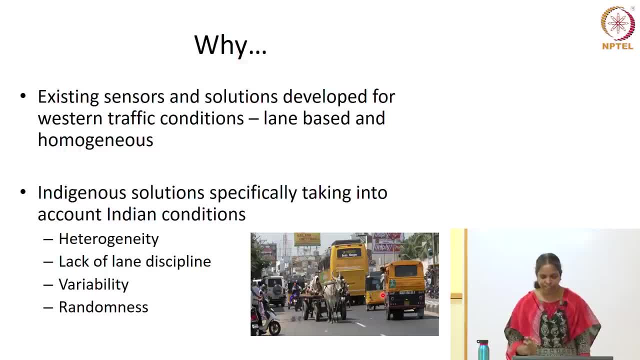 in whatever way. So how do we handle that? so any solution that is already available we cannot use, we have to kind of redo that, Okay, Okay. So this is the whole thing to meet this requirement of lane less movement. The other is heterogeneity. we have all types of vehicles. there are some 16 different types. 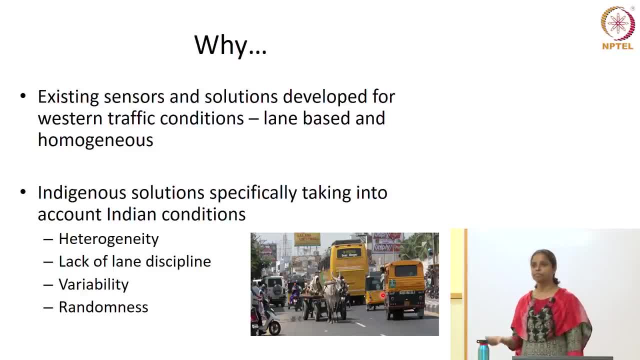 of vehicles that can be running on our roadways. So the typical US road. if you look, you have cars, you have truck the car, very small percentage of truck, maximum number of cars. so again, very simple way of handling. So, as I listed, heterogeneity is one chapter. 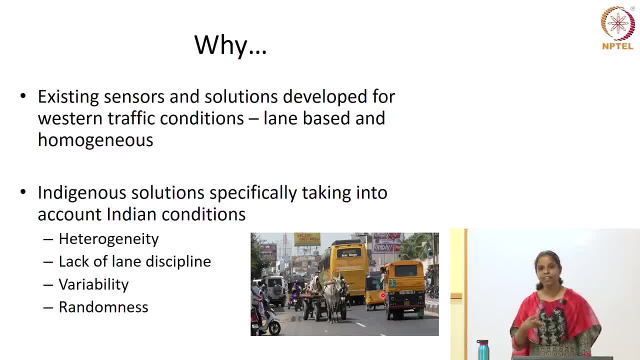 is one challenge. plain discipline is another. These two together gives you enough uncertainties. randomness. So any model which you develop should actually be handling this randomness than the actual behavior. So your thing should be able to take into account the stochasticity. 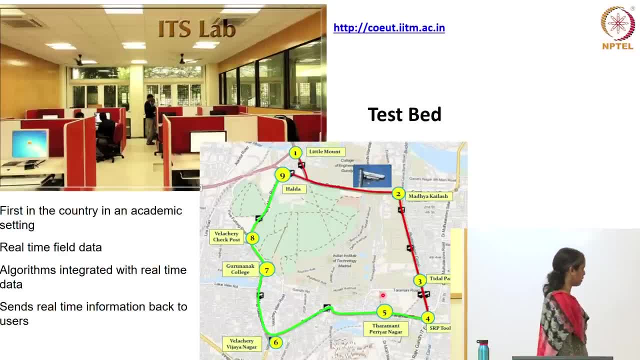 in the model. So this you do not need. you know what plain discipline is, So why I said that is? many of you otherwise may wonder: why should you do this? this is already done in other countries, right? Most of these solutions or most of these things already is happening. 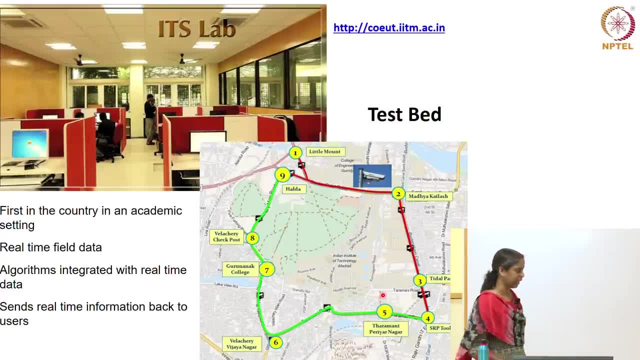 why do we have to? Because we have a unique way of handling. So, as I said, we have a lab and a test bed. Lab is just a place where we are receiving all the data. the test bed is the interesting part. So we have a 15 kilometer corridor around IIT, SP road, IT. 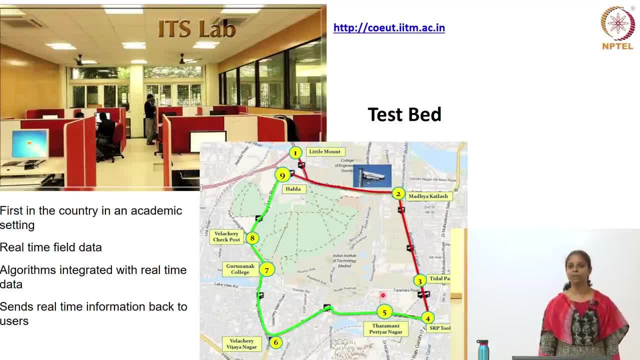 corridor. you may not be knowing, at least some of the Chennai's will know. So it is all the roads. So it is all the roads outside which are surrounding the IIT campus. The IIT is actually in that way So and we have kept enough sensors in those roadways. there are some I have. 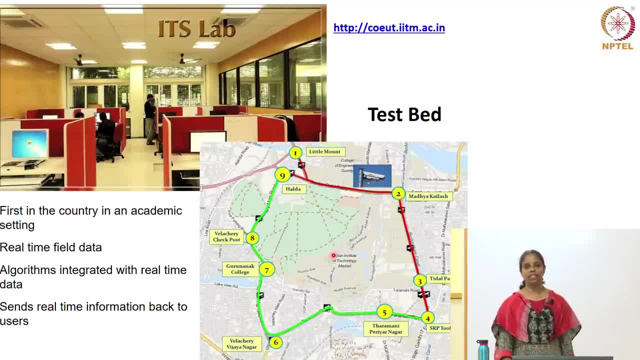 the details. So this is the first time an academic institution did that actually, even non-academic places where they do not have it. So we have real time data coming from field, we are processing it, we are having algorithms running, solutions being given. 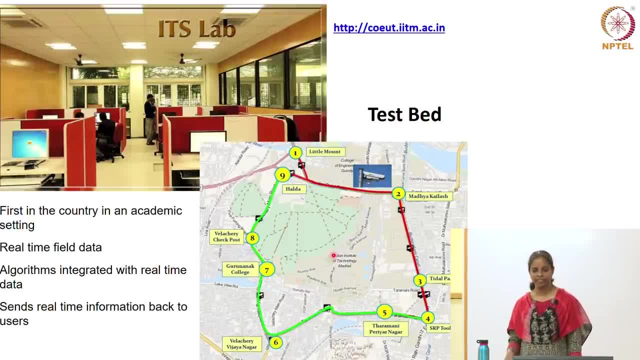 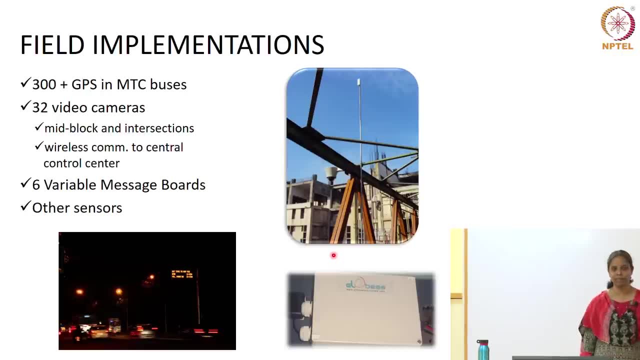 back to the user. So the complete They have. all this change over the death of people Results as to did not reduce. So all the services they have made there are increasing because there is no faster access. they wanted it greater, easier, more, faster information. 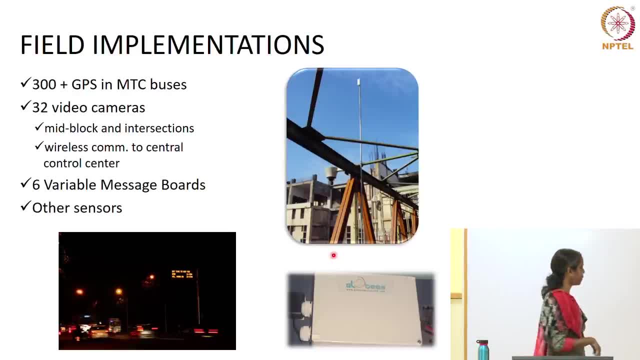 to be added to bus and then they force it to others not to run weer studio services like IIT railways, as you all are familiar with transports. is that right Bus and poi bus that was there is we use the same system as cathodes. 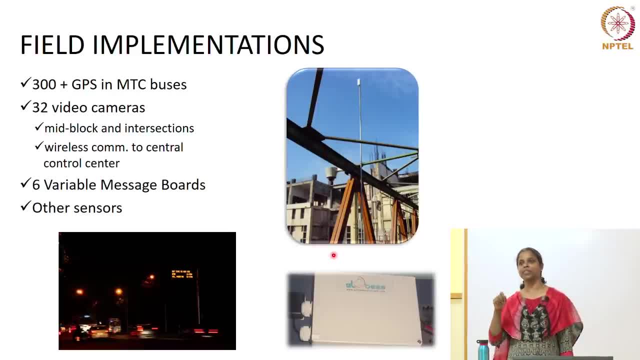 And these connections. we have implemented these small corridor. What are all the sensors? we have around 300 MPC buses with GPS sitting and sending the data to our lab every 5 second or 10 seconds. We have around 32 video camera relaying their 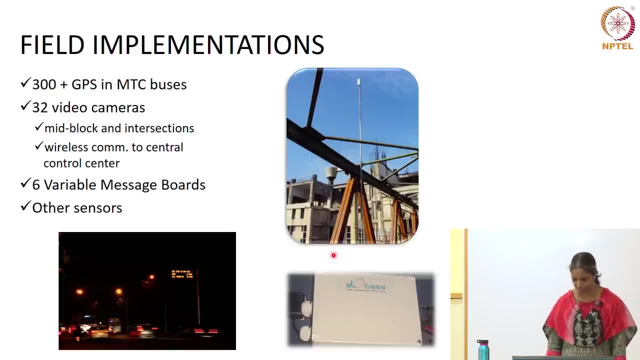 feed to our labs. So then we have message board, which we have installed in the field, which gives information back to the users, and there are other several sensors, also being this, which I have enlisted. all of them are sitting in the field and sending us data. 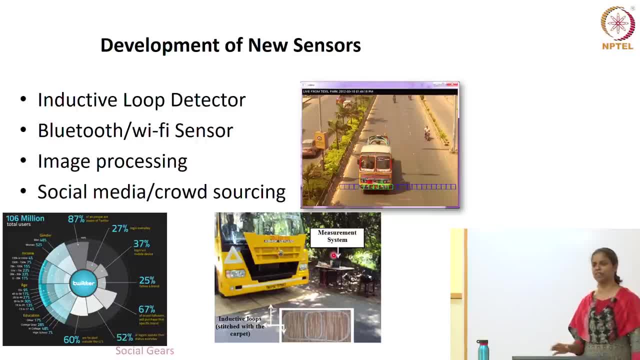 And many of the students were involved in developing sensors. So this is not purely a civil engineers work alone. we collaborate with electrical engineers, mechanical engineers, engineering design. I have a slide showing all the collaborators. So we work. so I usually joke about this. if you, some of you may be feeling very bad. 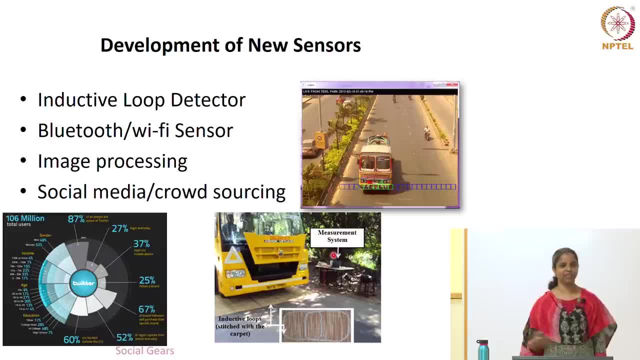 that you wanted to be an electrical engineer or computer science engineer and you ended up engineering. These are ways in which there is no fixed territories. these days, it is all inter-decisionary. nobody stops you from working in any of the topics you want. 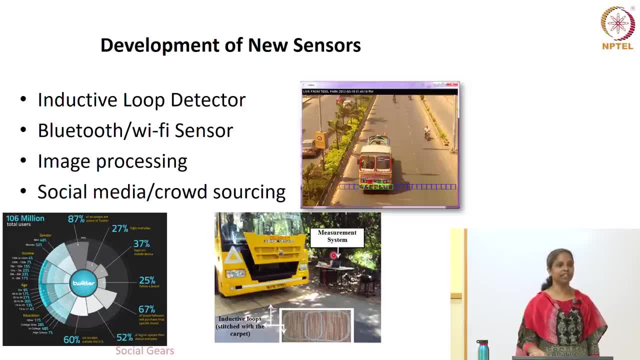 So this is one of the areas in which lot of my students work with electrical engineering faculty, developing sensors. We have developed at least four different sensors which are working and giving information in a much larger scale, So this is a much better way than any of the available sensors. 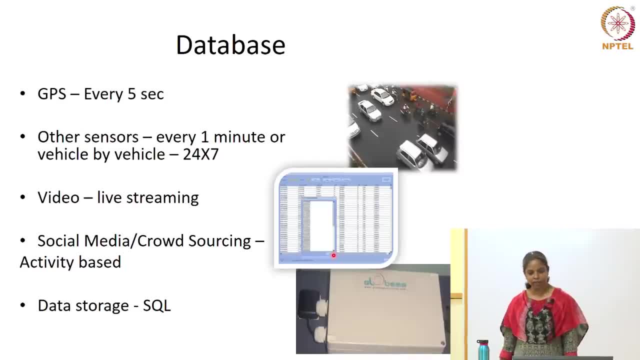 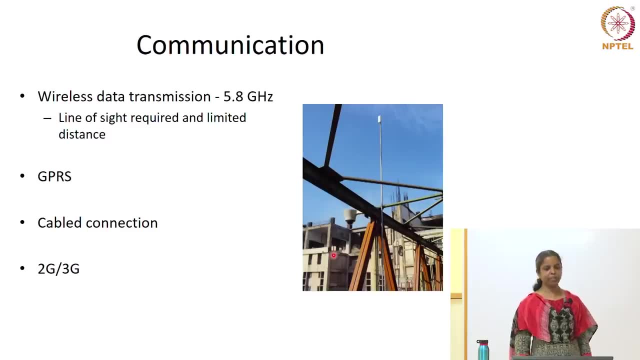 Details I do not have time so I am not getting into. So obviously we have a good database, lot of data that is coming from all these sensors And communication. we are using various technology: GPRS, wireless data transmission, regular wired connection, 2G, 3G modems, etcetera, etcetera. lot of modeling that happens, which 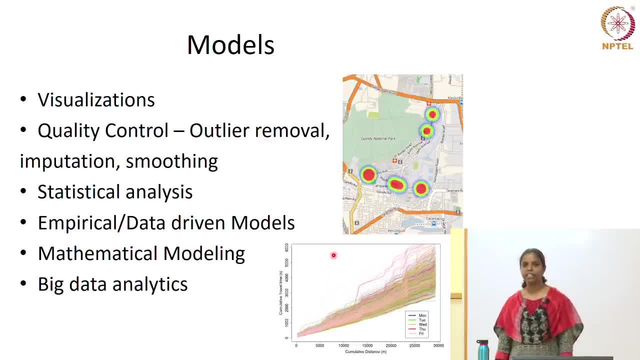 again, I cannot get into details, Ok, But starting from very simple empirical models to, you know, mathematical models, to data analytics, are all are happening. So, depending on your interest, you can pick what you want to try out and then you will do it. 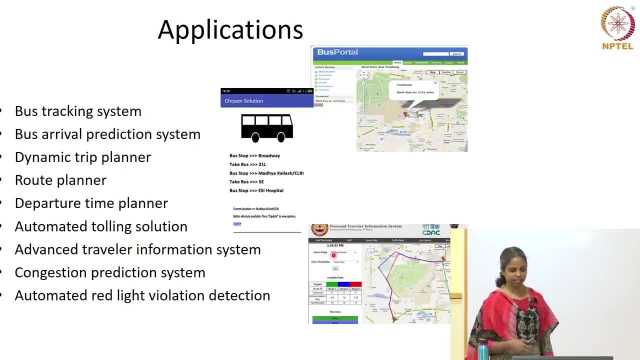 Some of the applications which we have developed include bus arrival prediction system. What you see as the picture there is actually a live system where you can go. click on the route number. It will show the bus stop. You can click on the bus stop. 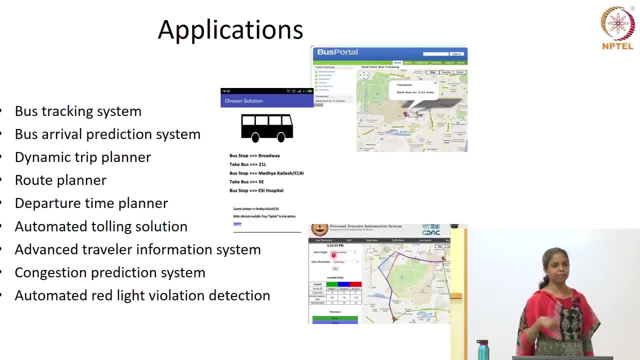 It will show when the bus will come. So if there are multiple bus routes, it will show. these are all the route numbers. which one you want, you can click and it will show. So there are many solutions that were developed after I said, most of them are undergrad students. 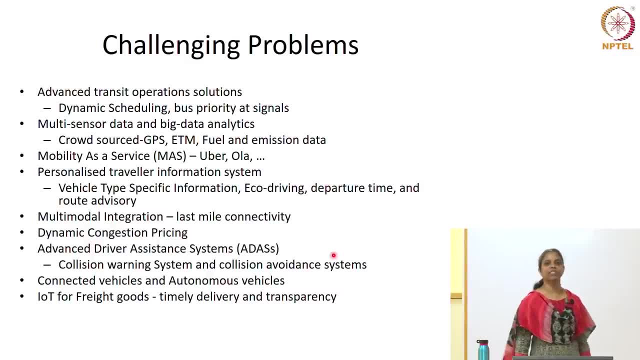 work And I will stop with what are some of the challenging problems, which are often which, if you get interested, you want you can work on. For example, dynamic scheduling. No city is doing that. Ok, They all have this fixed schedule saying every 20 minutes one bus has to leave, or every 30. 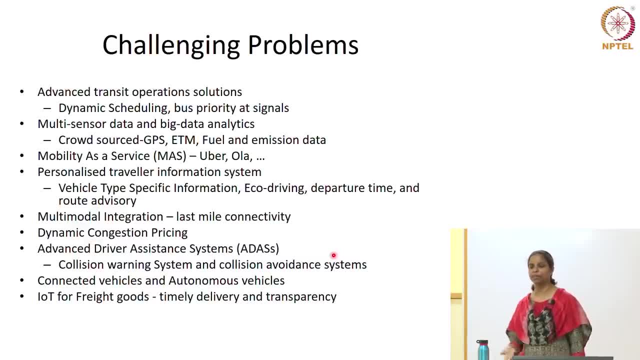 minutes one bus has to leave. It does not make sense. Peak hour: you may need more off peak hours you do not need. So how do you handle this in a dynamic way, depending on the actual traffic situation? How will you schedule? Each of this problem, as I have listed, is an interesting, open problem which can be worked. 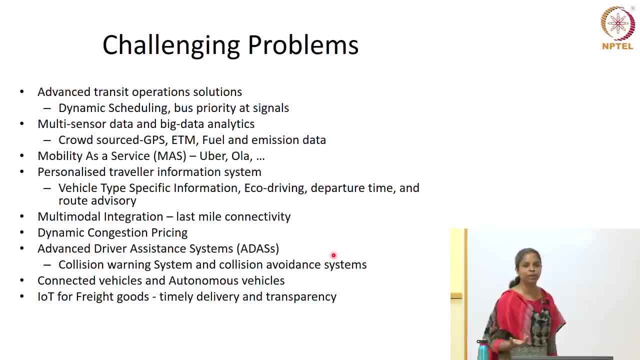 on Mobility as a service. It is a clueless problem. It is a very complex problem. So how do you handle this? How do you handle this? These are all very complex problems And even if you do not have a different bus route system, it is a completely different. 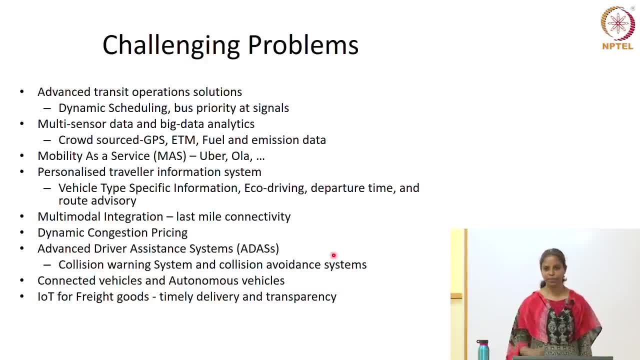 from a bus, completely different from a traditional taxi service. So how do we handle the scheduling, the routing, How do we do that? All those are, as I said, interesting problems. I do not know whether I will skip this, as an undergrad student may not be of interest.